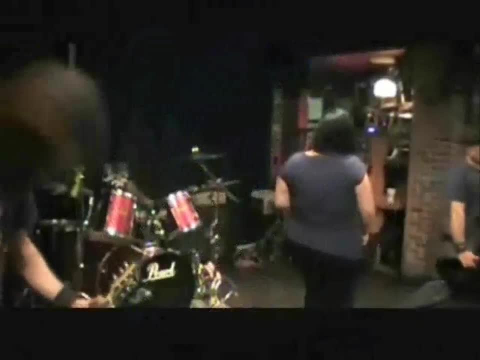 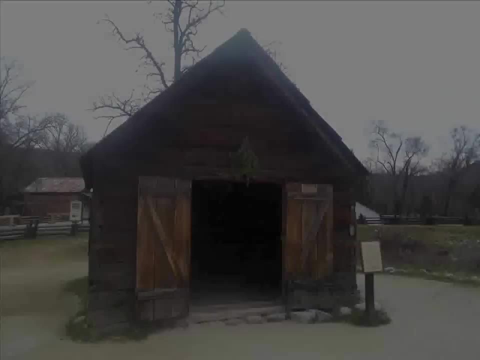 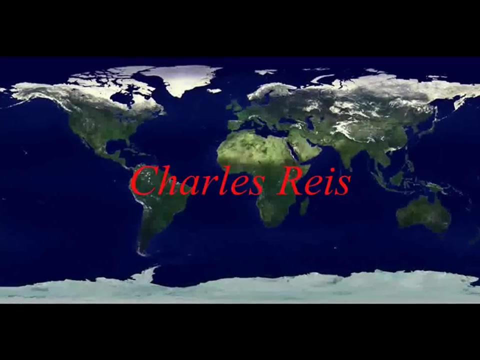 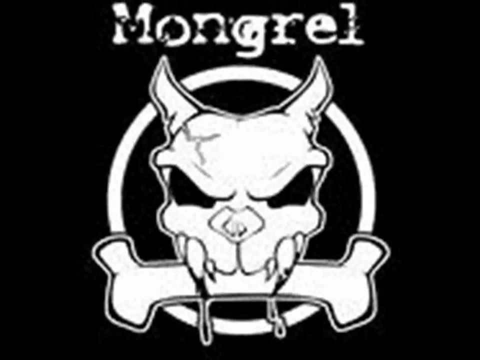 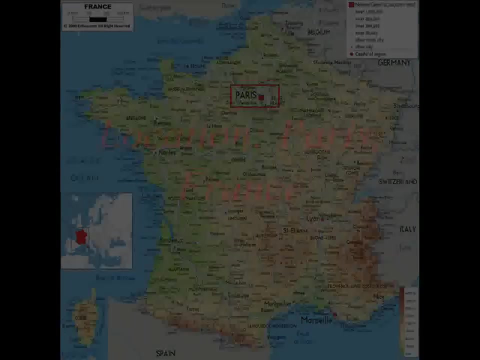 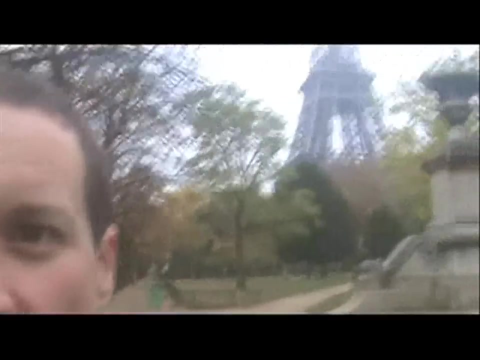 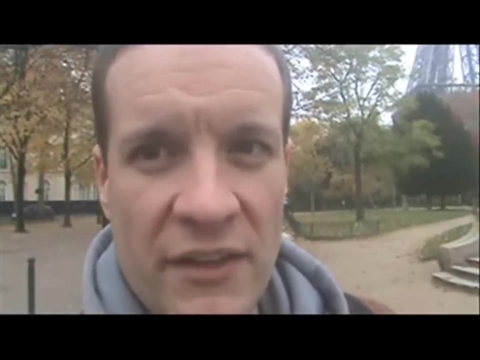 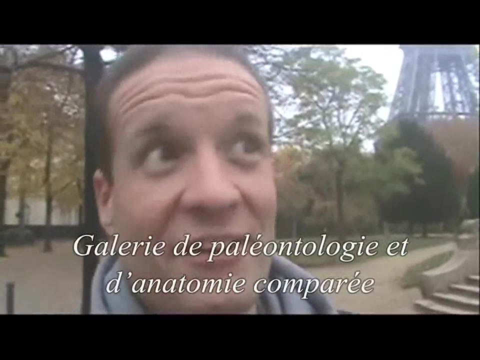 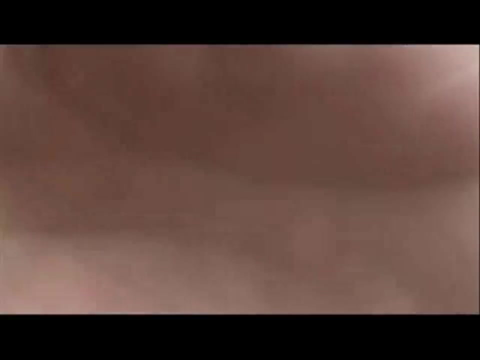 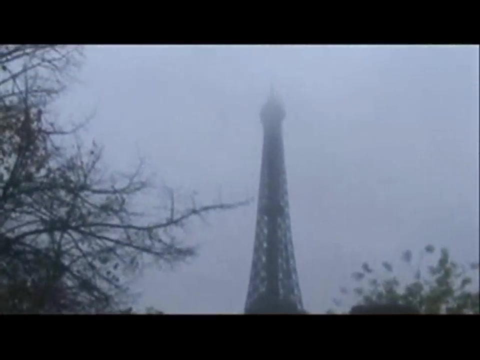 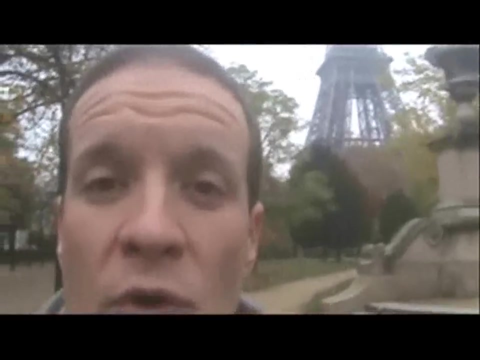 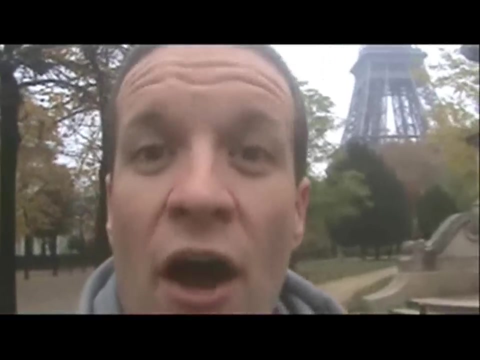 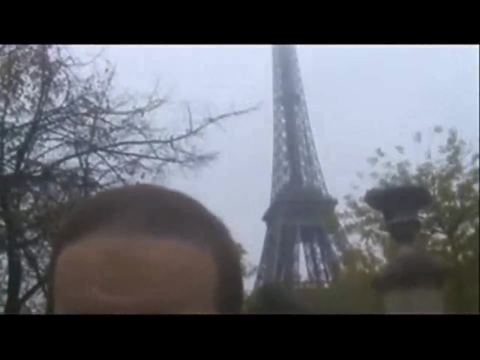 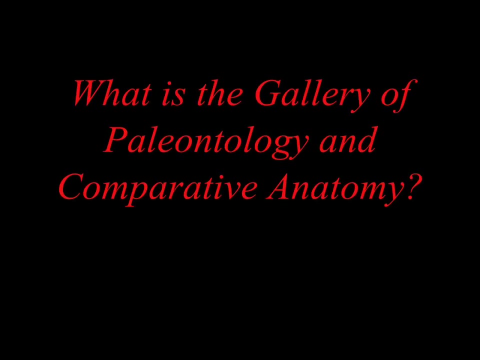 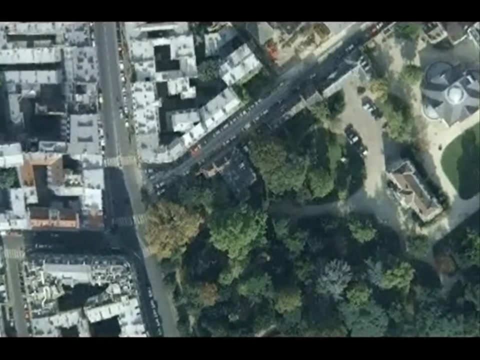 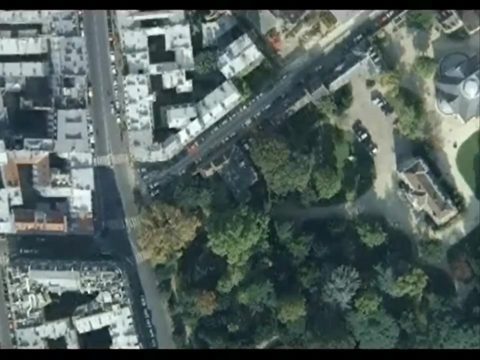 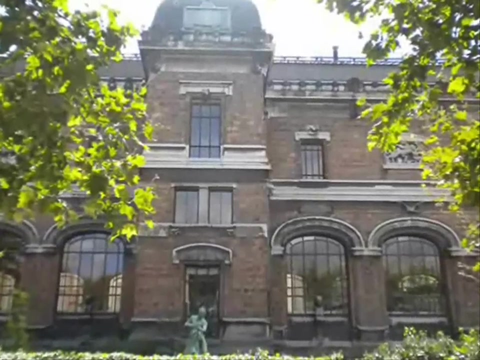 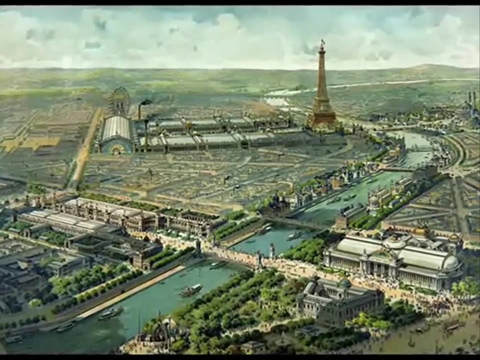 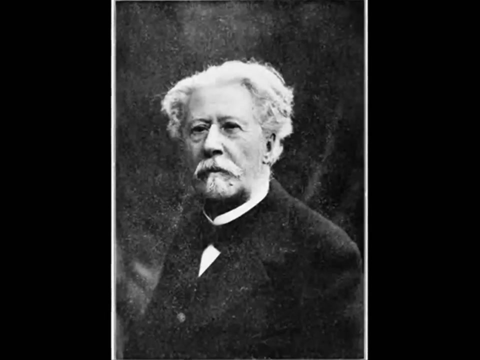 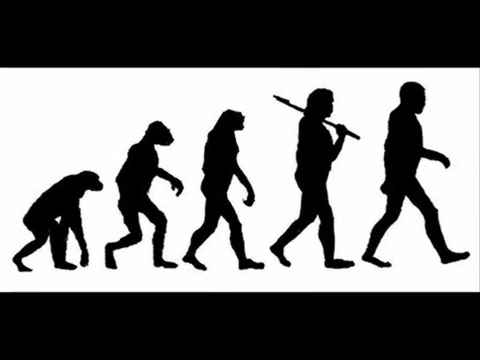 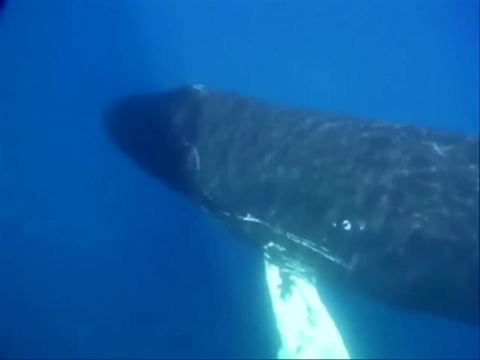 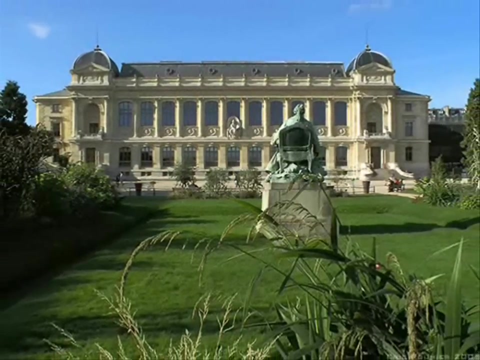 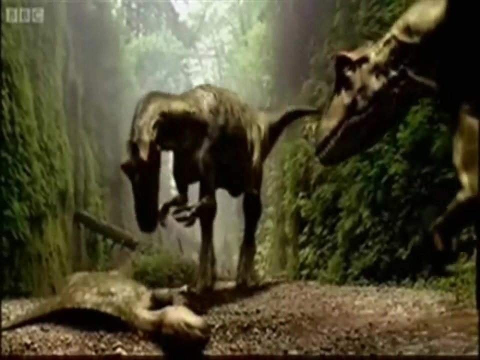 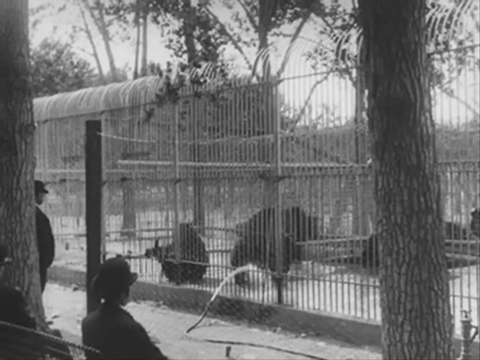 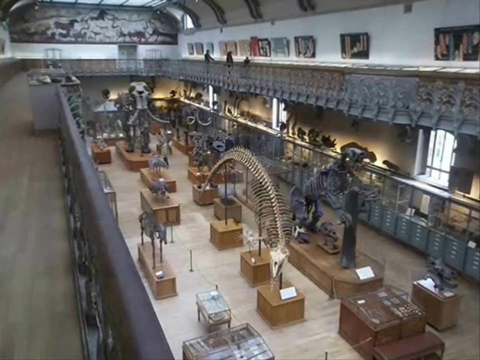 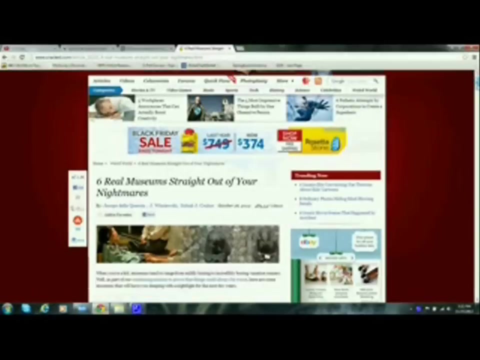 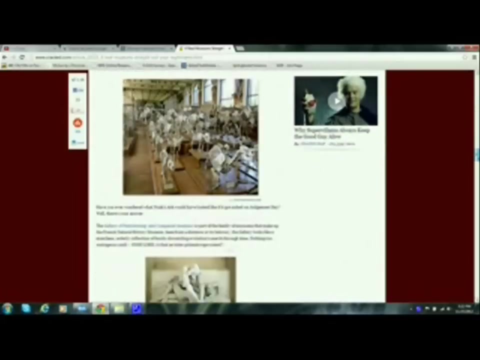 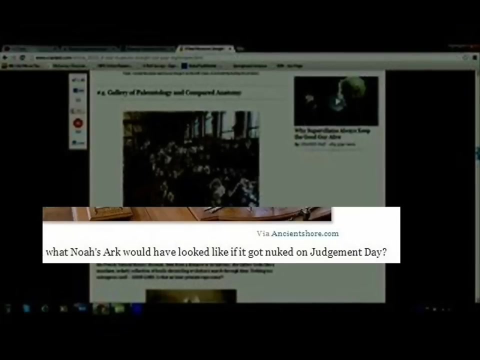 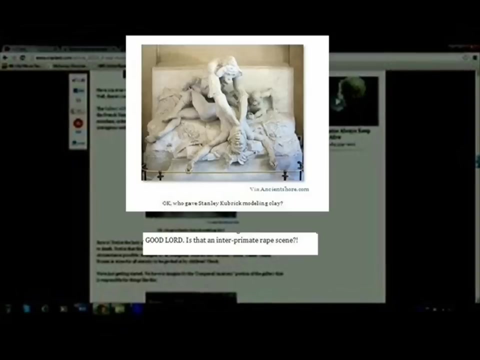 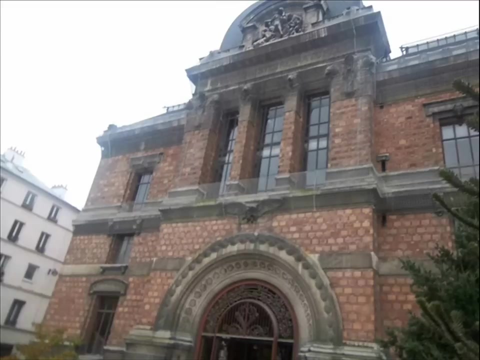 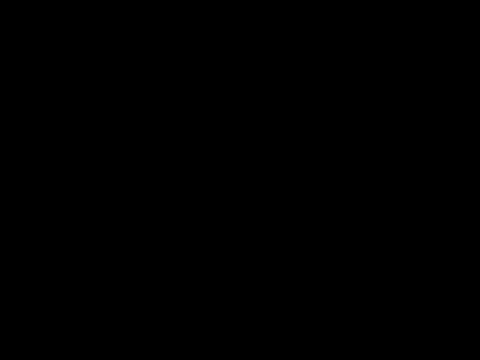 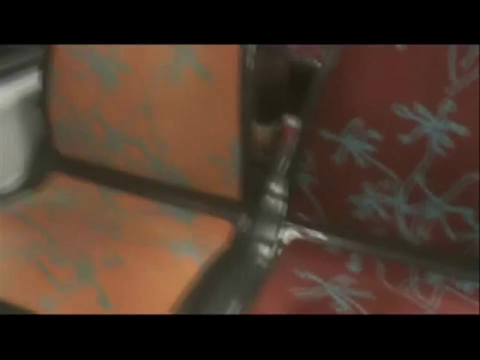 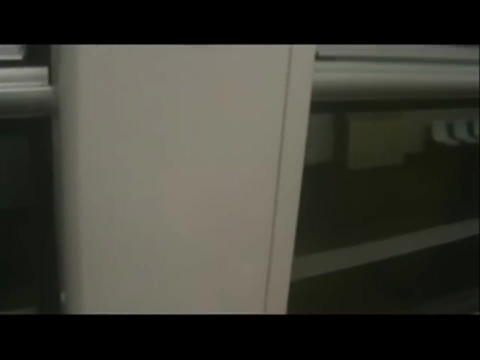 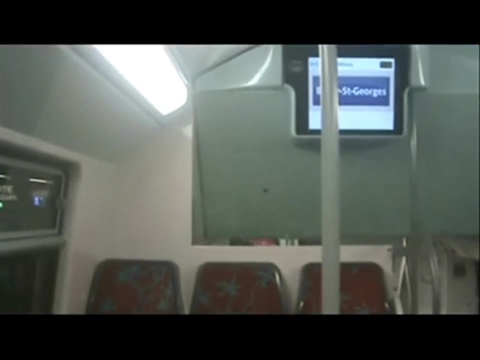 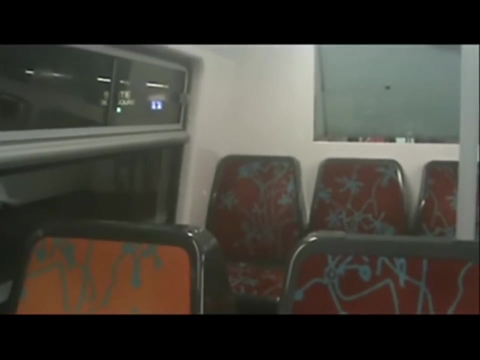 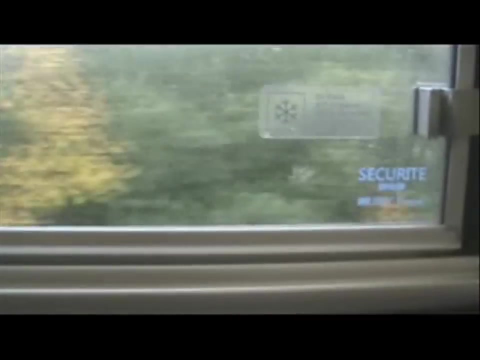 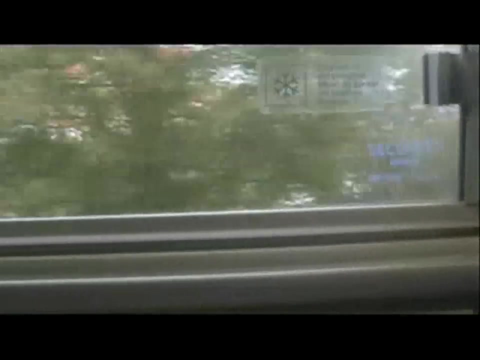 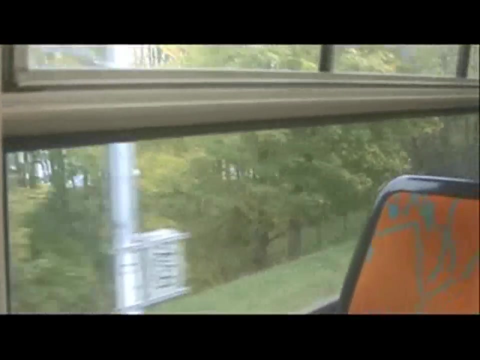 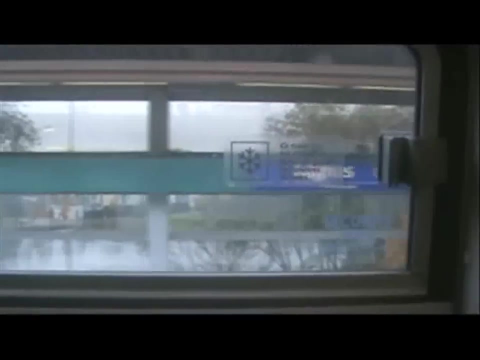 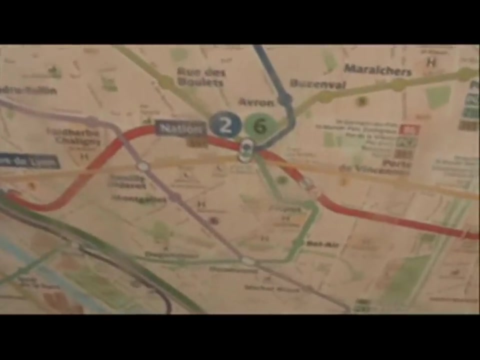 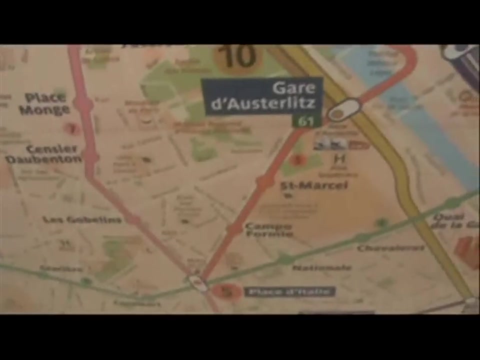 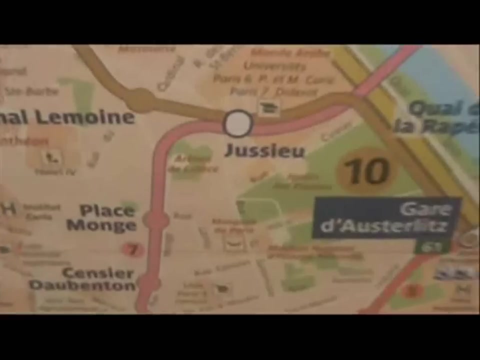 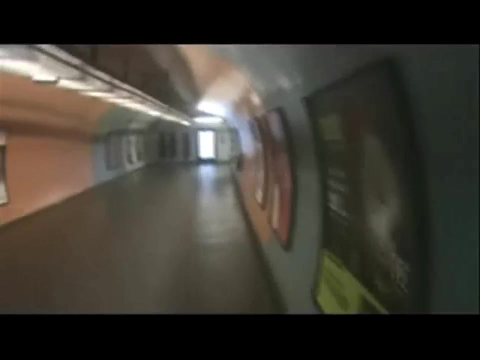 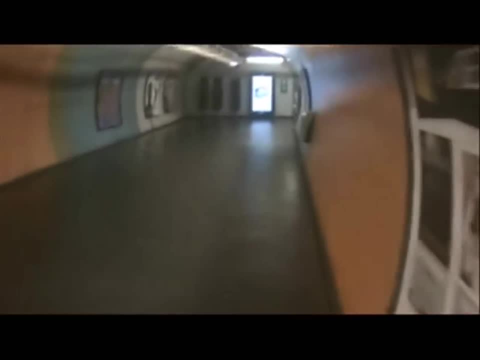 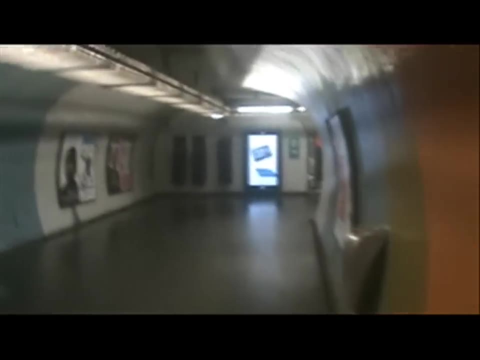 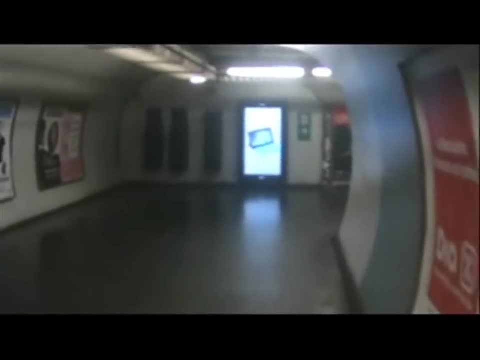 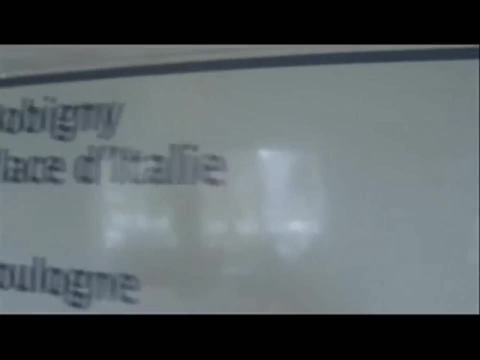 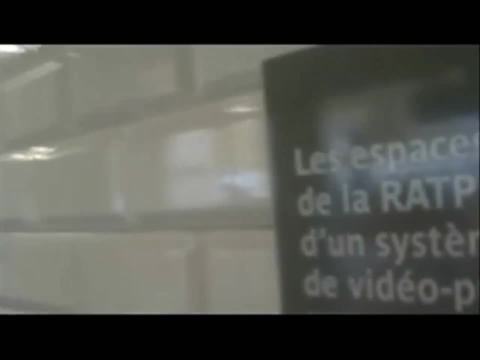 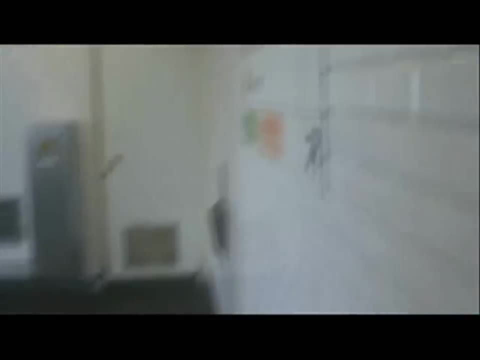 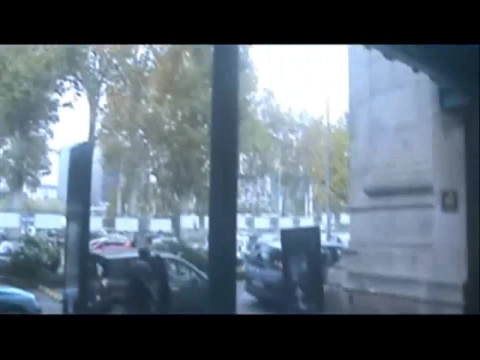 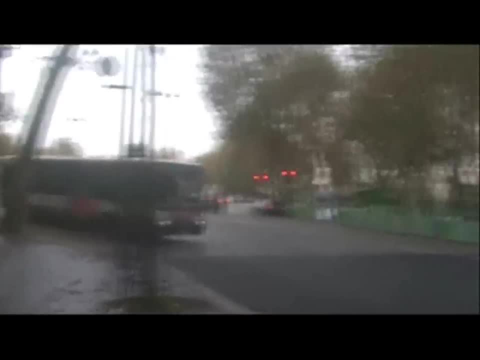 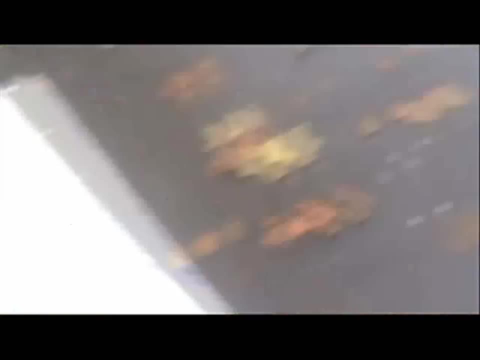 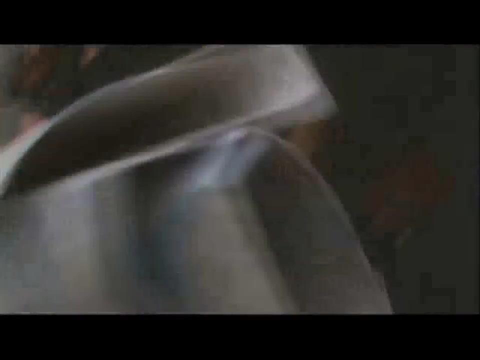 Okay, now I'm walking street level. Here's Paris. There's a Parisian bus. I'm going to, according to the map, let's see. Yeah, get a map. You're going to need a map, especially for some of these locations. 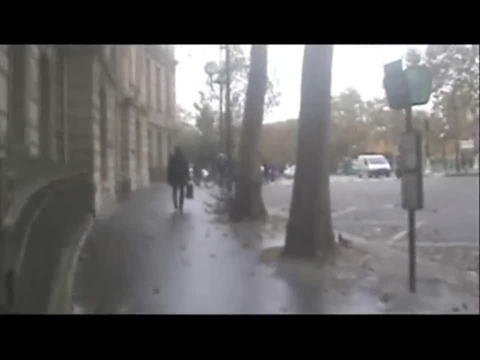 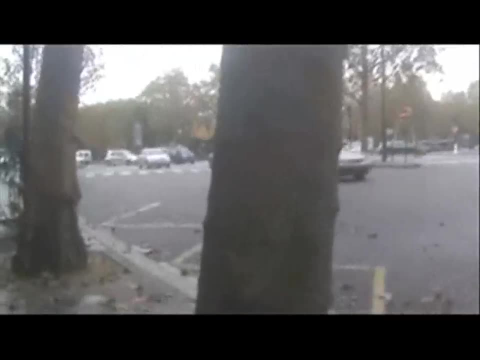 But according to the map I'm going to head down this way. Hey look it, It's a policia. No, that's in Spanish. Anyway, almost there, I think It's not too far of a walk, but 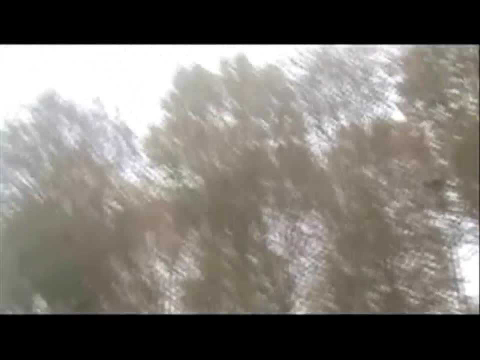 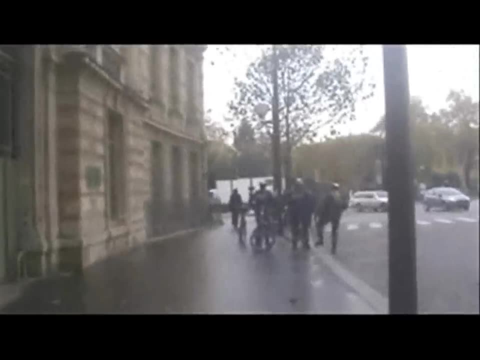 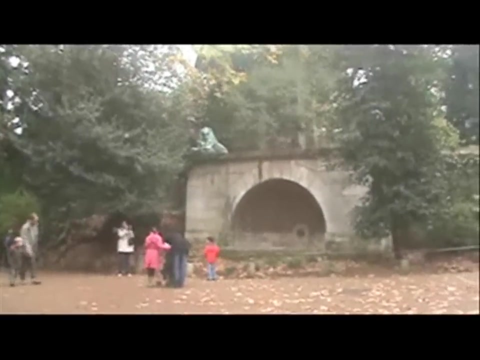 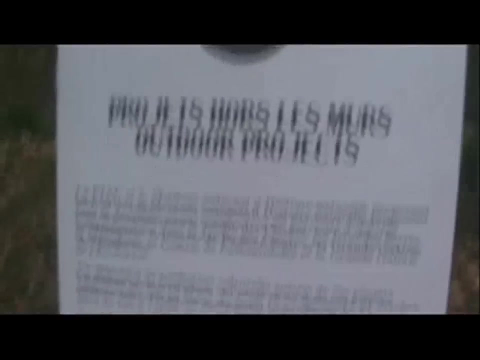 It's better to walk in Paris. You're going to miss out on all the architecture, And it's actually kind of a nice day out today. Okay, keep on going. Next time, hopefully, I'll be at the museum. Well, I'm in the grounds area where the museum is. One of the entrances is located over here. There's actually a few of them, And so you get these and then you get stuff in English. I think I got to head down that way. 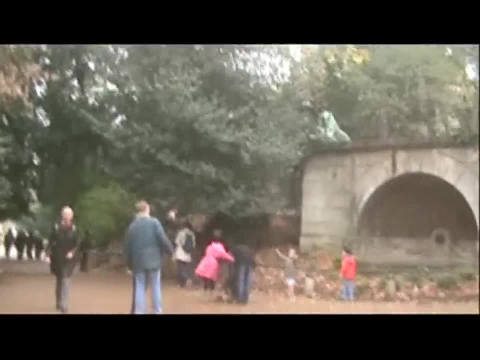 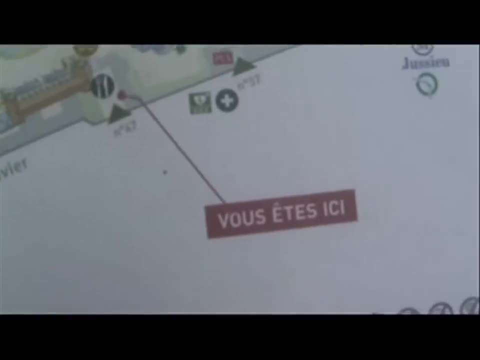 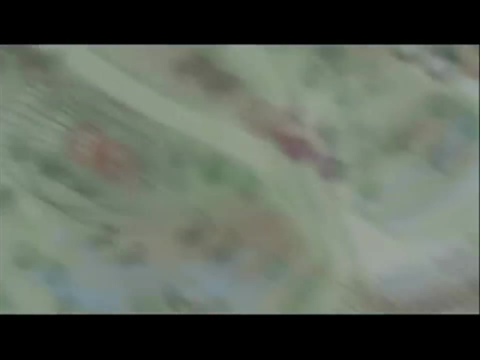 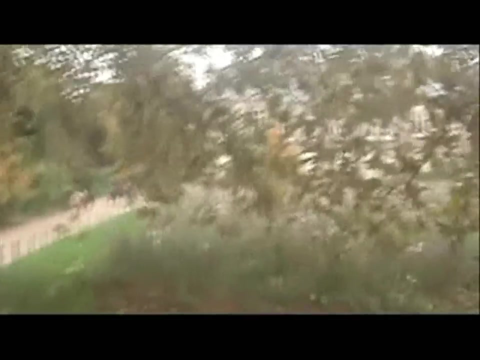 Kind of a nice view. It's a nice looking park, So wish me luck if I get there. Well, I found it. I'm assuming you- I know that's like you or something, or you know something- You are here. We'll just say that I'm so bad with my French- And the museum, the entrance is up here, So I got to go and well, you know, even though I haven't got to the museum yet, it's still nice to stroll through the park area. 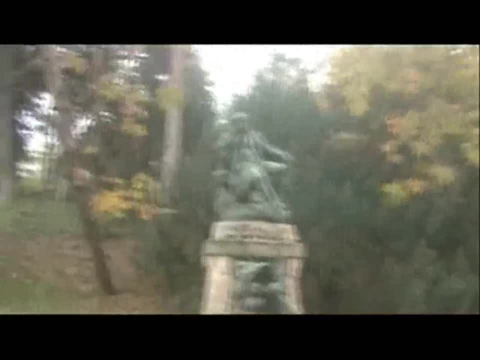 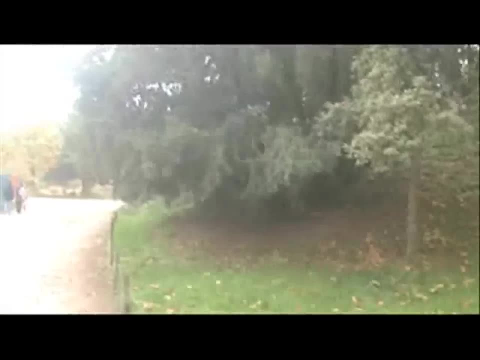 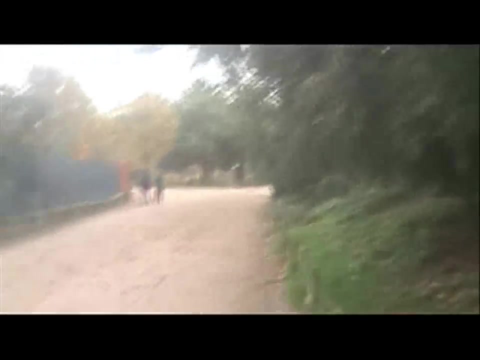 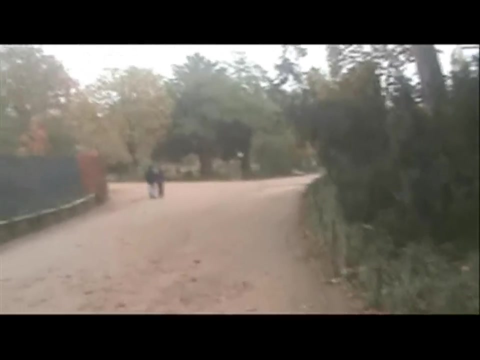 This is more like a science park, A lot of like museums on history and evolution, because they believe in evolution and plants. Okay, I think I'm heading in the right direction. I kind of know where it is now, But I feel bad for any. I like more sympathetic now for people who come to America and don't speak English, because it's hard And I know a little bit of French, but not enough to hold down a conversation. 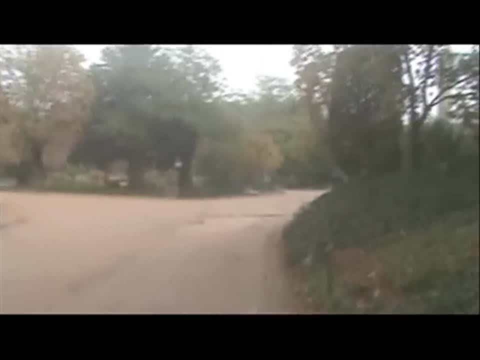 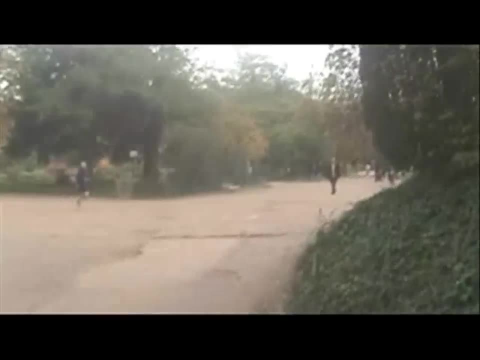 So it's been a challenge, but that's okay. You know it's France, They don't speak English And I knew what I was getting myself into. So I am tired. I might take a rest later, So off to the museum. 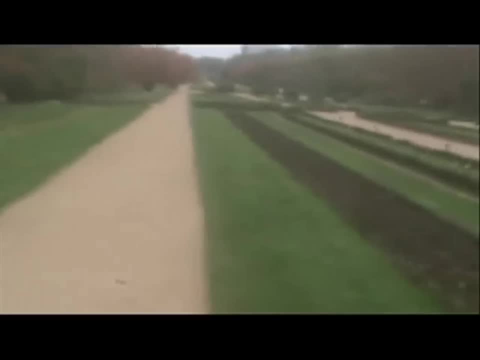 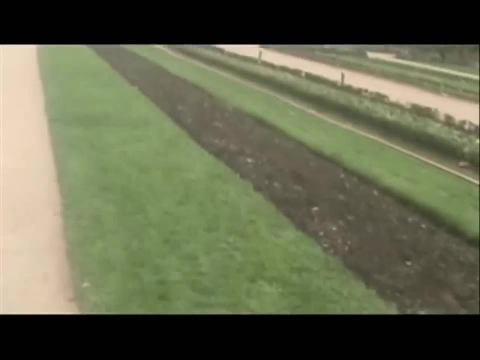 Well, I'm still trekking along. This is actually. I wanted to turn the video on because this is actually a very beautiful spot. If it wasn't fall it would be even nicer. you know, more blooming of the flowers and trees and stuff. 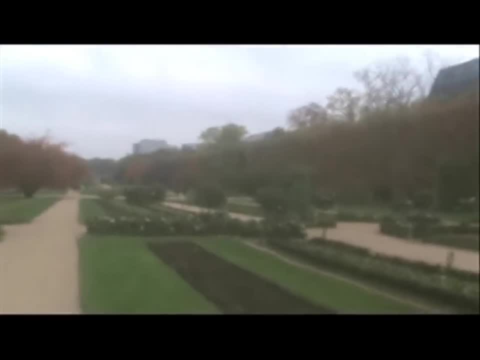 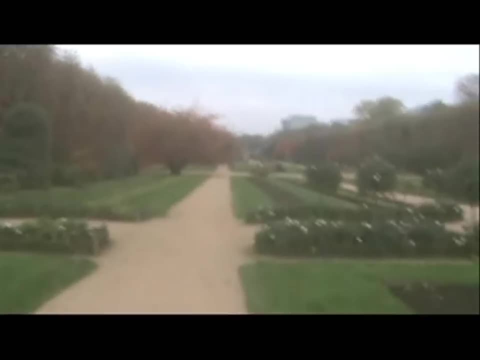 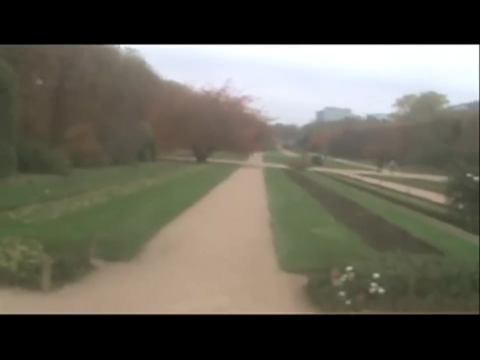 But I think it's the building down there. Of course, then again, I was. I've been wrong already, That's okay. Isn't that all part of like exploring? Just trying to find your way to the places you should have? Me and Steve, even in America, we get lost trying to find the most simplest of locations, And with the added challenge of the language barrier. Well, as they say, c'est la vie. 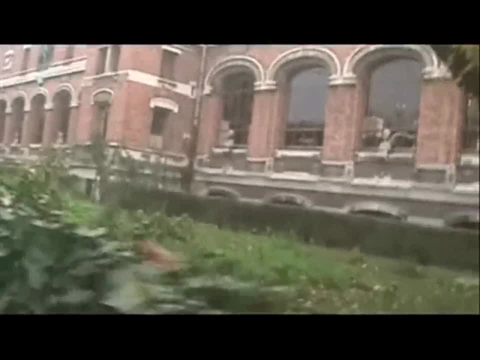 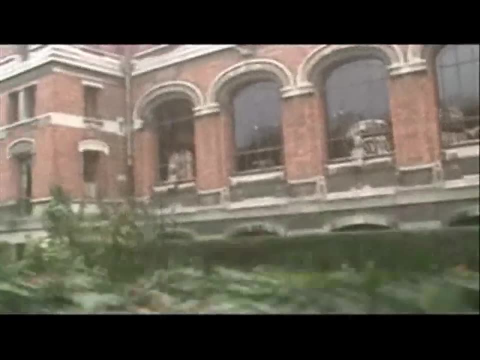 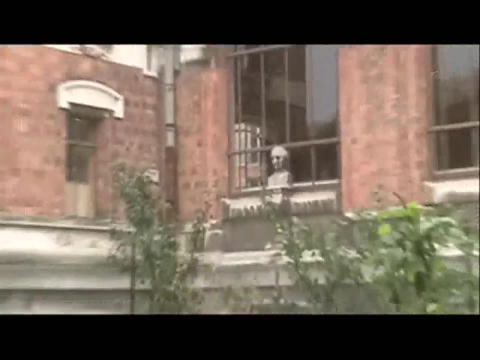 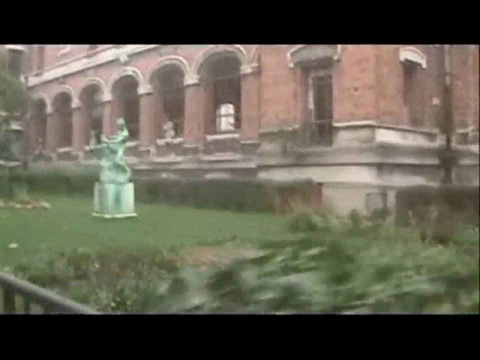 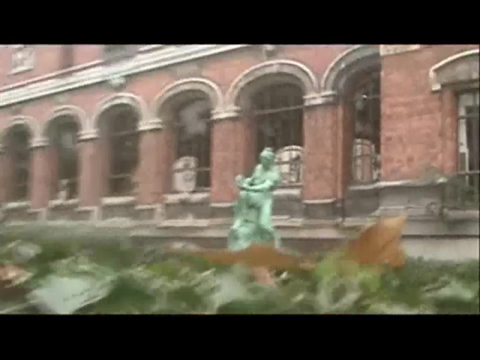 Well, welcome to the museum. I want to show you the outside. I can see the bones in the inside And, yep, this on crack is considered the museum, one of the top museums for your nightmares. And these statues right here. they look kind of like their eyes are bleeding. That's kind of creepy. It's definitely an old building too. I don't know who's that, But at least I made it. I'm surprisingly. you know, I'm definitely walking longer. I'm not having too, too much difficulty. 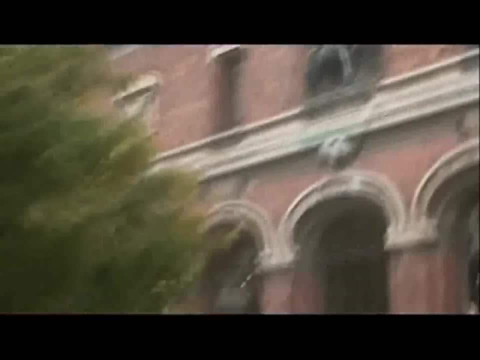 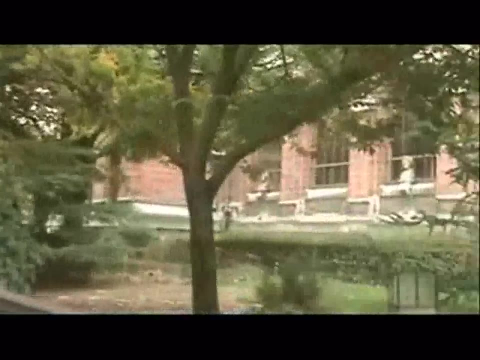 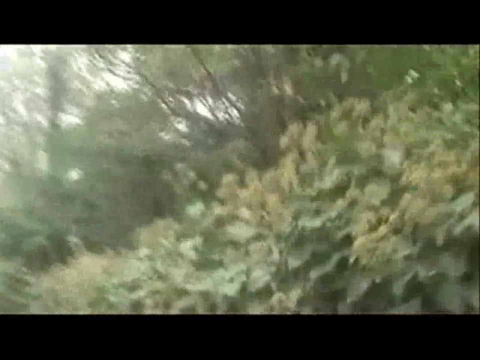 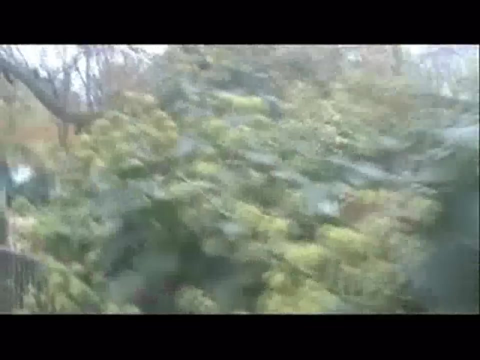 So getting to where I want to go, Nice. So next time I turn on the video, I shall be on the inside of the museum once I pay my euros- And yes, by the way, don't pay in American dollars, Don't be like you take dollars. They don't like that very much. Not that I know that from experience, I'm a little bit too smart for that- But I know people who have done it. You don't do that, Okay. Okay, one more score shot, I swear then we'll. the next shot will be on the museum. 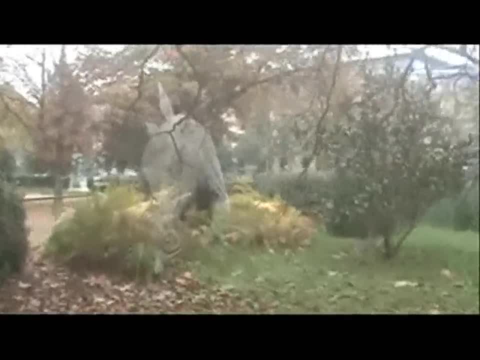 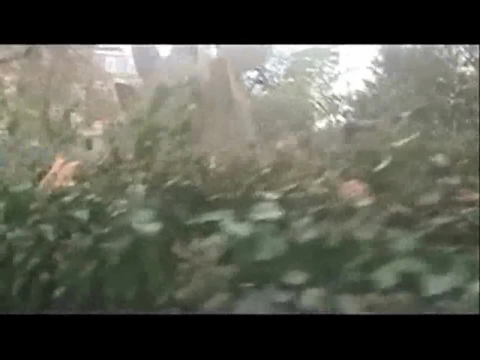 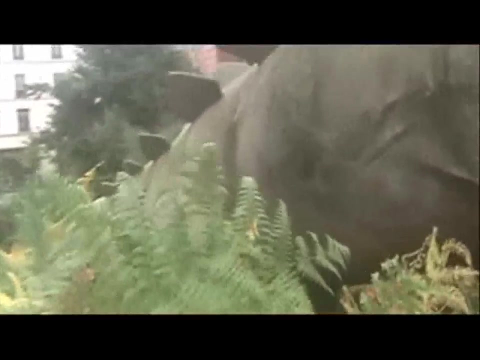 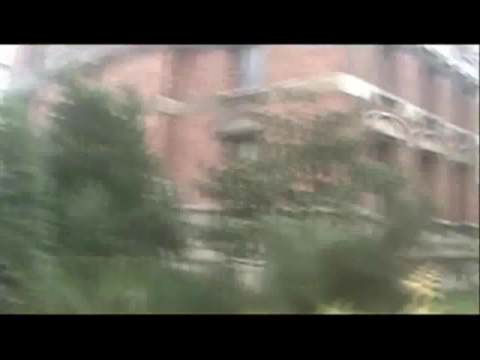 I want you to see a dinosaur, a stegosaurus. This is how I know I'm in the right spot. besides that, the fact that I can see bones in the museum windows In land before time. he would be named spike. The entrance is over here. that's the tegatoris, the entrance over there. 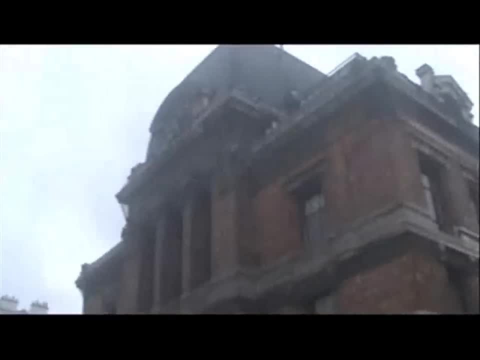 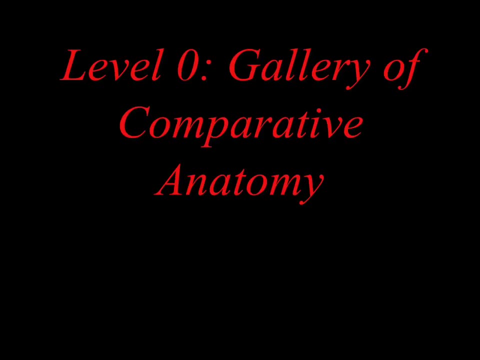 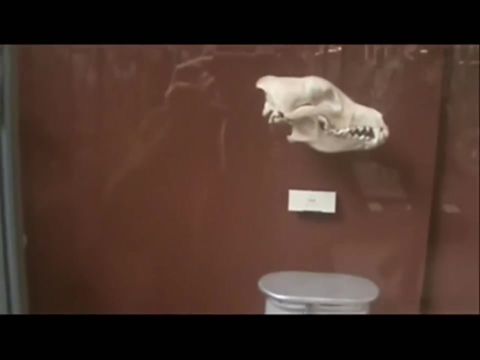 I think, and um, we shall be in my way. actually it's a kind of a creepy old museum too. I wonder if it's haunted. Oh Well, I'm in the museum, finally paying, luckily the lady. Generally, the best thing to do is say bonjour. 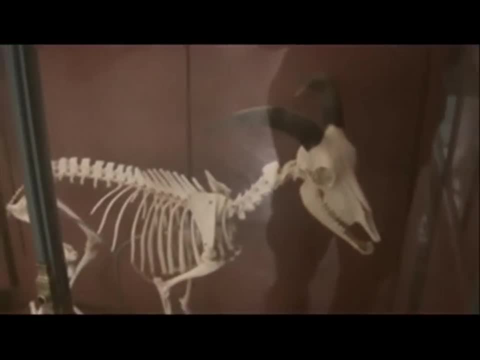 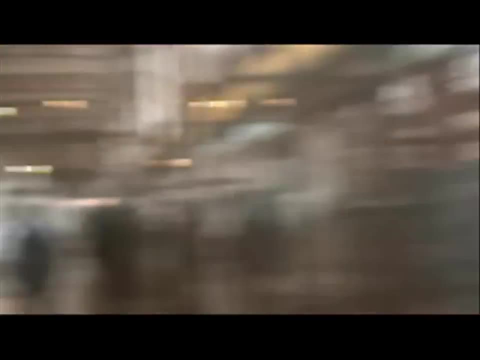 Madame or Missouri polybu in clay, and they tend to be a little bit much nicer because you just don't want to assume everybody speaks English. it's rude. Okay, I can see where the creepy factor comes from. There's a skinned man right over there. 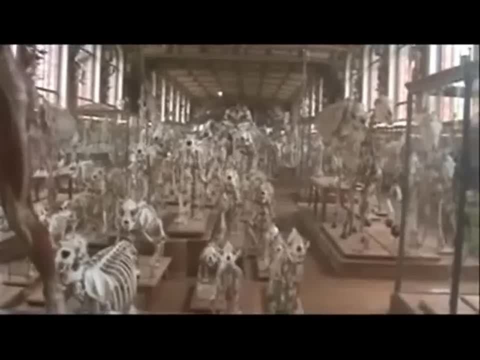 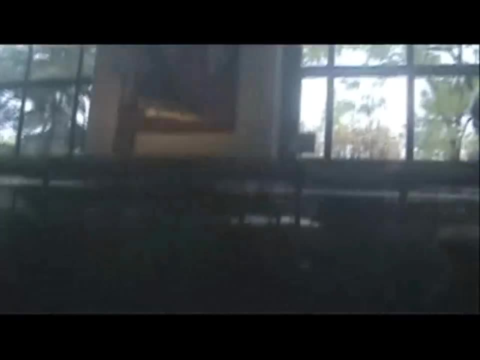 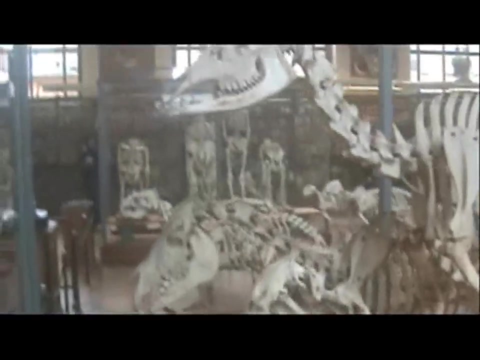 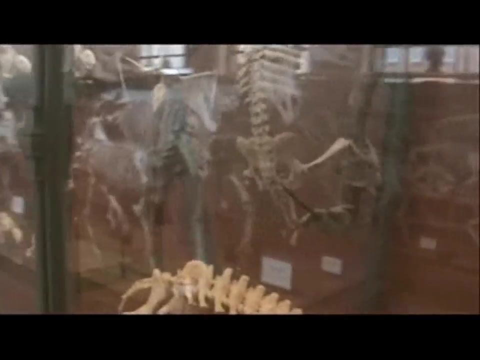 It's like Hellraiser. okay, Yeah, see, that's why the museum is considered of your nightmares. There's awesome, but like skeletons everywhere. so Here we go. I heard you. So like the museum of like dead rotted animals. makes it wonder, gets the animal. 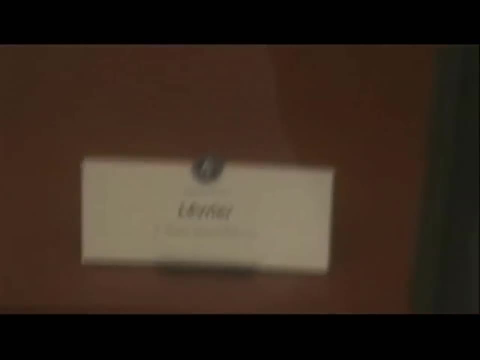 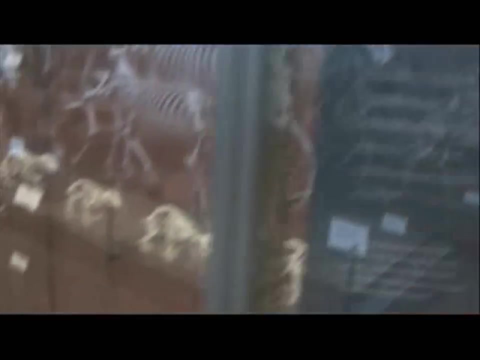 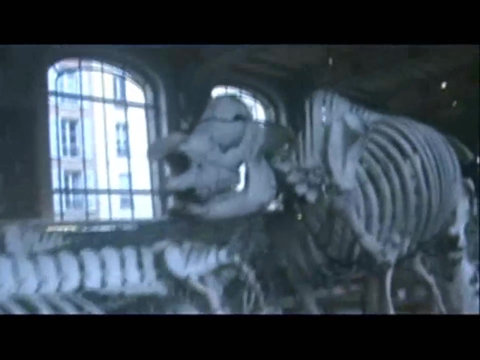 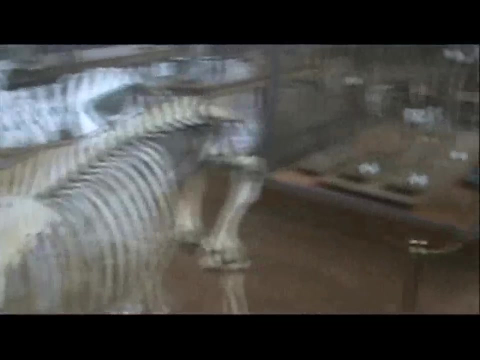 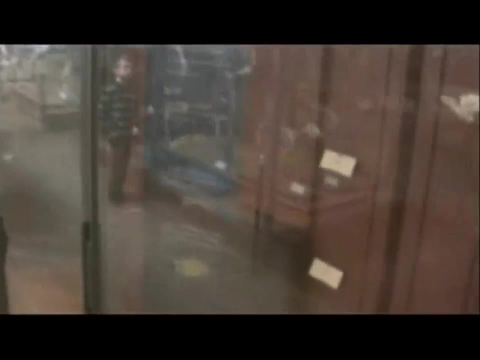 I'm not sure what that is. I'll have to look that up Some time. maybe wolf or something That looks like a bat I I? I don't know if they're real or not. I'm assuming some of them are. I'm pretty much going to be going through this quickly. 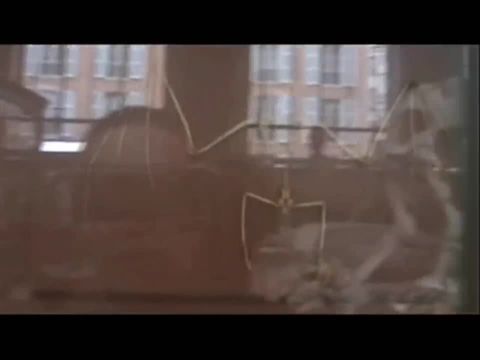 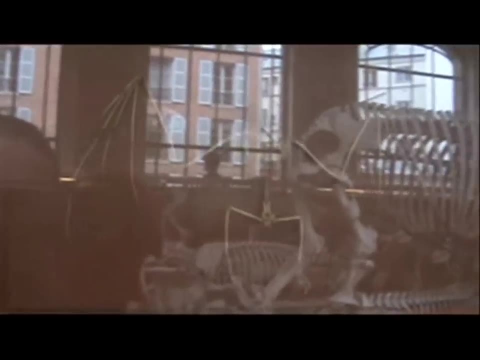 I can't read nothing. Oh, that's a bat. Let me get it. I want to see the bat. I'll have to take a picture of it because of the glare, I'm not sure if you can kind of see it. 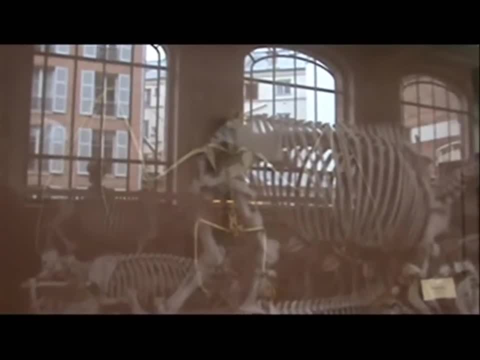 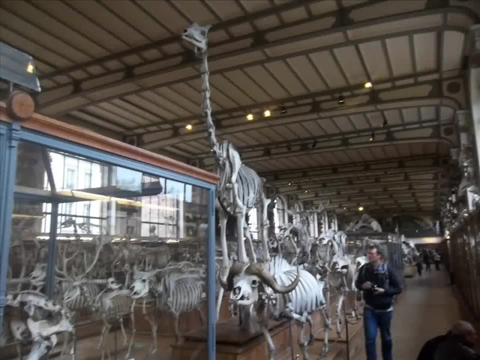 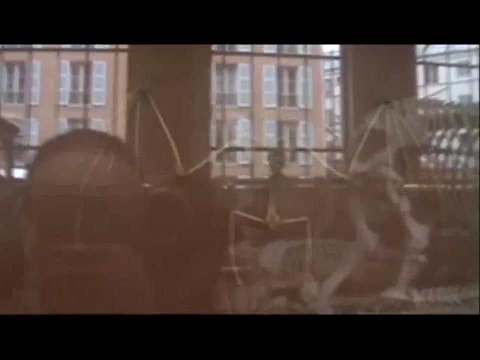 I'll see if. maybe, if I take a picture it'll be less of a reflection. Well, I tried to take a picture of the bat. unfortunately, at this little party It didn't quite work because of the reflections that you see me and outside and stuff. but 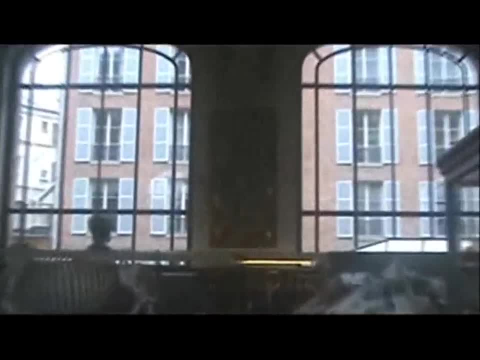 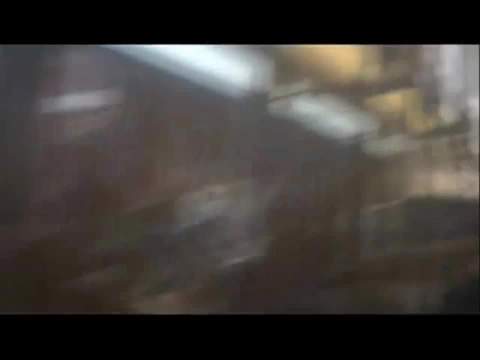 it's creepy. There's a lot of little creepy things all over the place There. I have no clue what the hell that is. And look at this: It's a dead frog. I'm thinking: Nope, nope, nope. 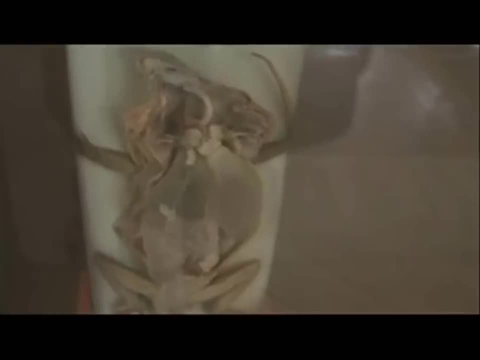 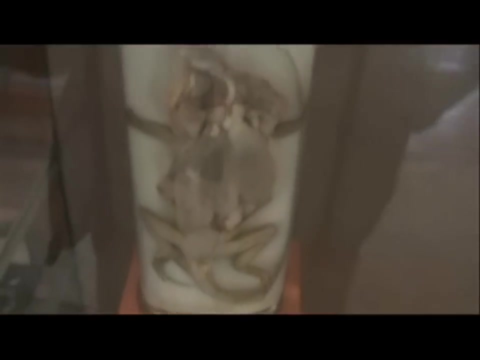 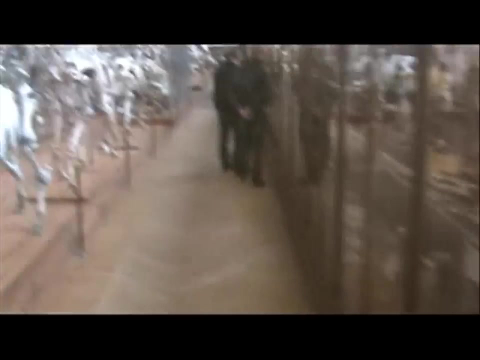 Lizard, Lizard. It looks like an iguana or something. Yeah, no need for ghosts in this little video adventure. You just need to look at all the bones. I like this one over here. I'm really liking this one. 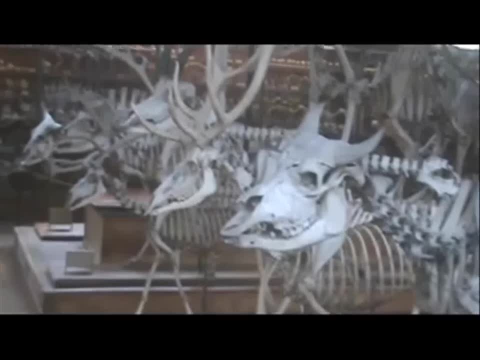 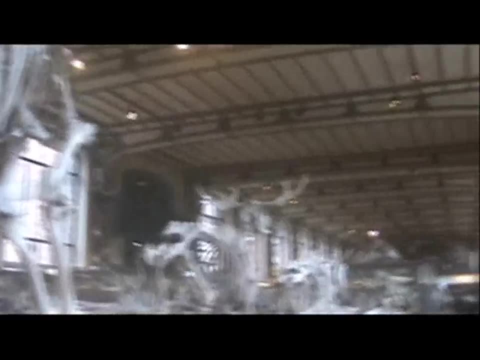 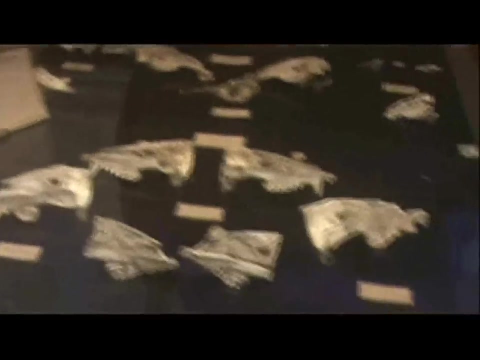 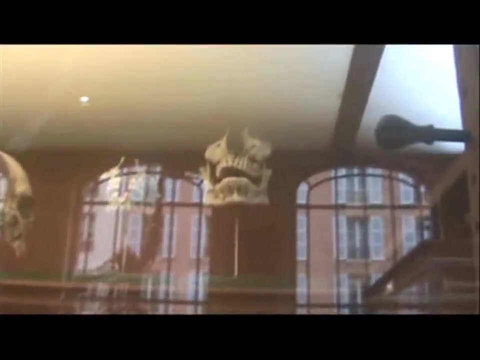 You can't jump over And I think there's a little giraffe. Damn, You don't really need to know French to come in here, Just come in here. and Oh, is that a human jawbone? It's a skull. 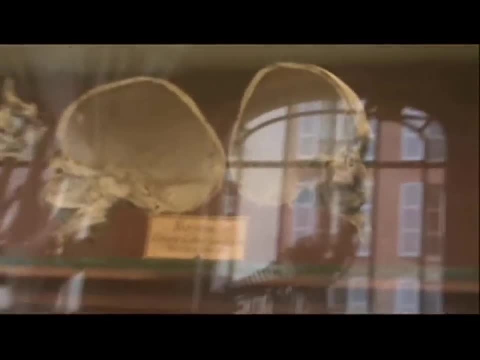 After I'll have to show you the statue out in the middle. That's probably when we come towards the end. I want a picture of him because I'm going to call him Steve. Oh, Steve, Steve, Steve, Steve, Steve. 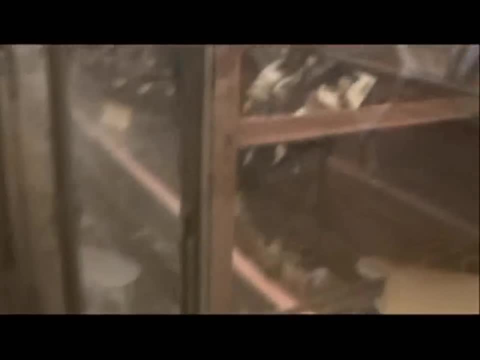 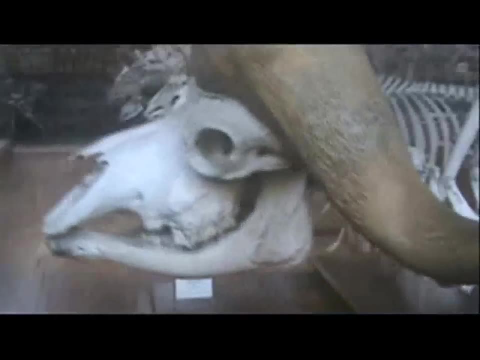 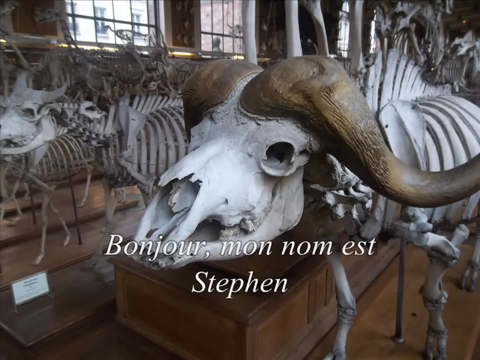 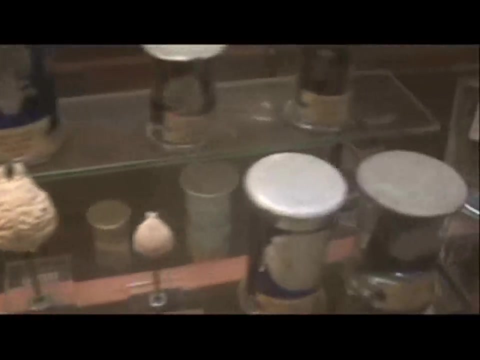 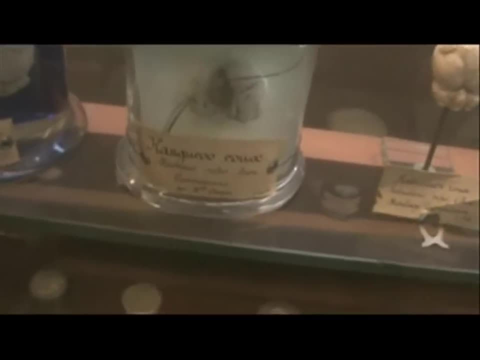 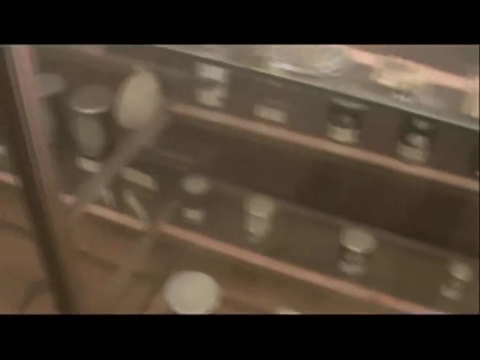 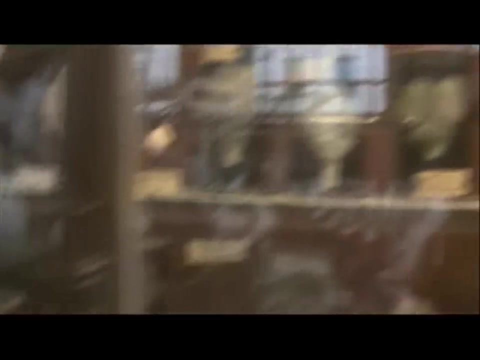 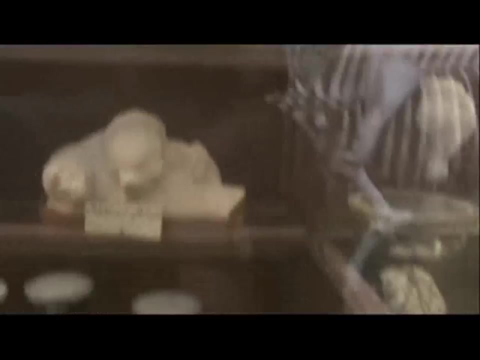 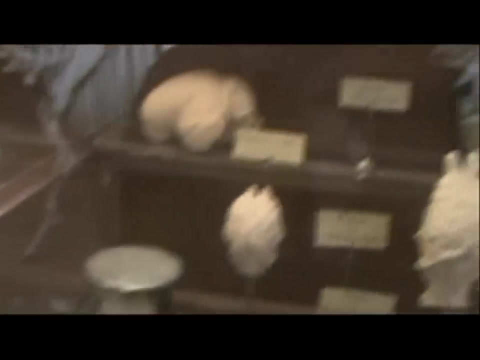 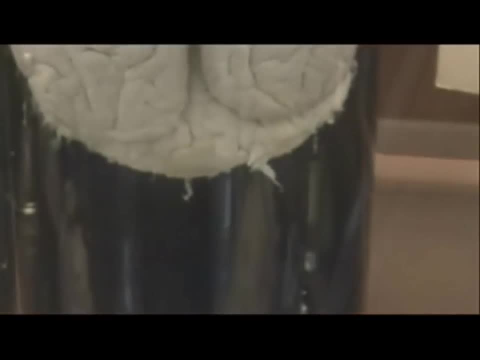 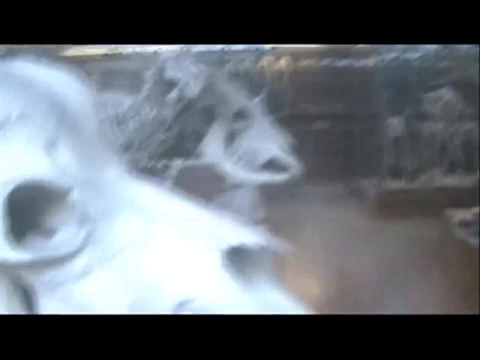 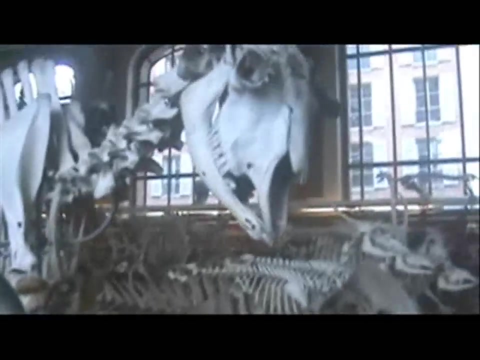 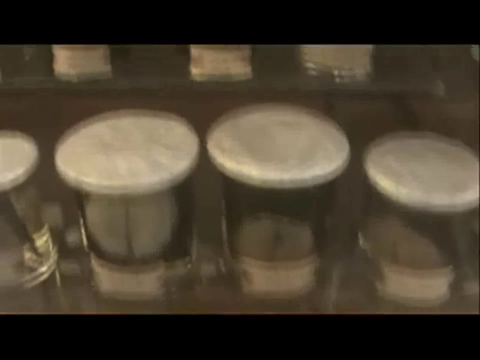 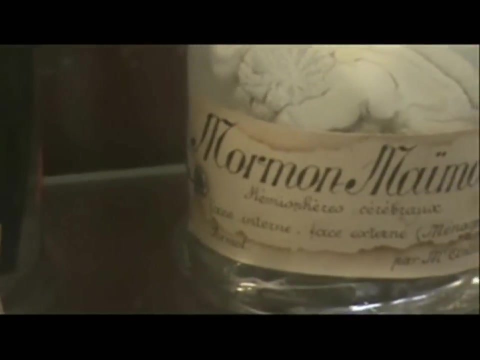 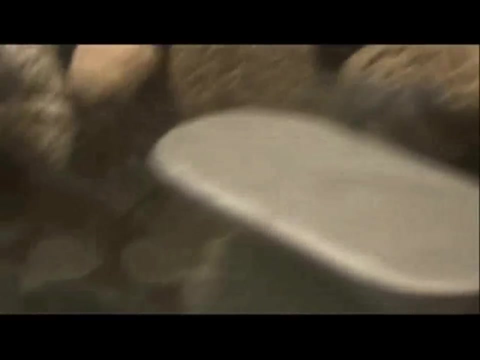 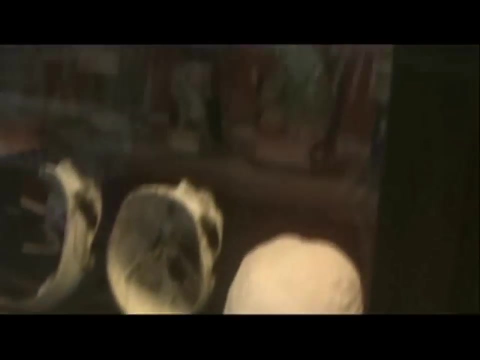 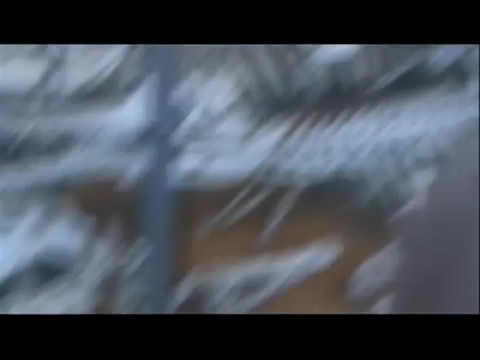 liquid state, so I'm assuming they're kind of real. There's more animals, yeah, brains. oh, for a minute, what is that mormon mormon brains? Oh, that's some mormon trains. oh, that's a mormon train. oh, that's a mormon train. 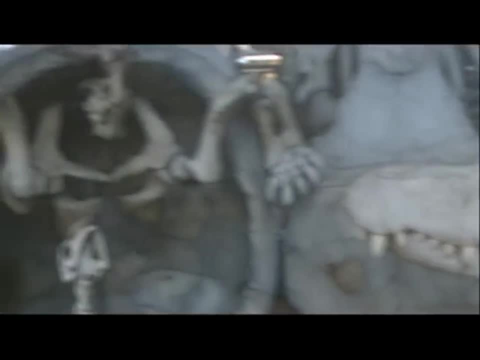 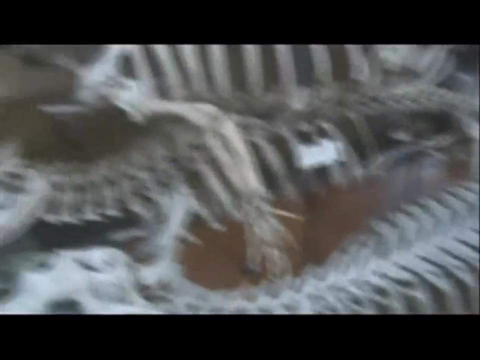 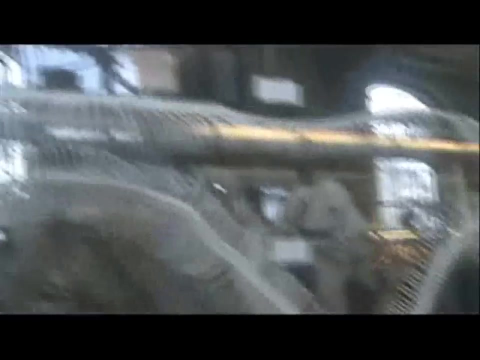 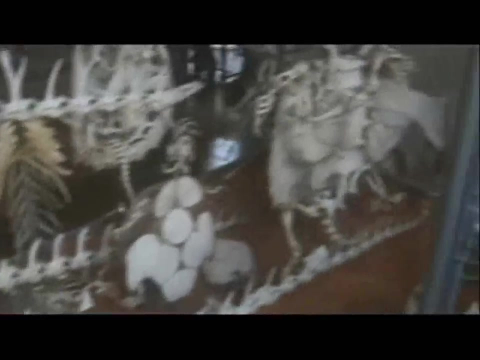 These five animals. Boy, you can take the skin off, that's gonna give you. oh, it works. Yeah, but some of these animals are even more scarier. this is a snake, or, uh, anaconda- this is the second floor- more like ripped up animals. 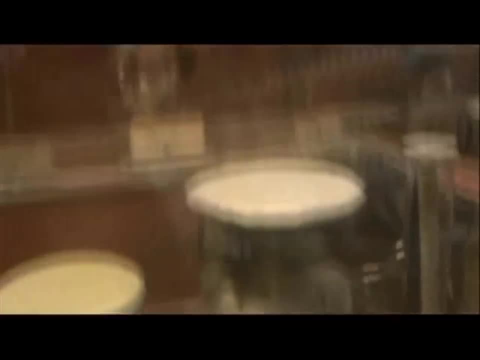 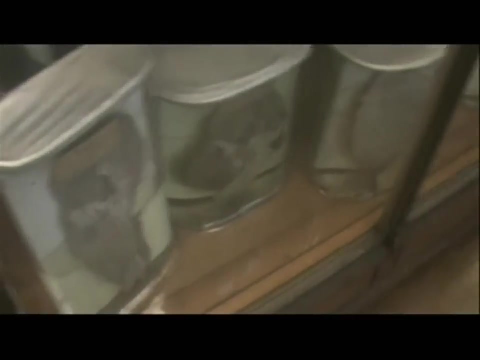 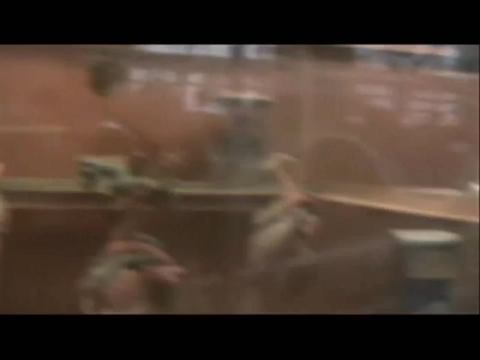 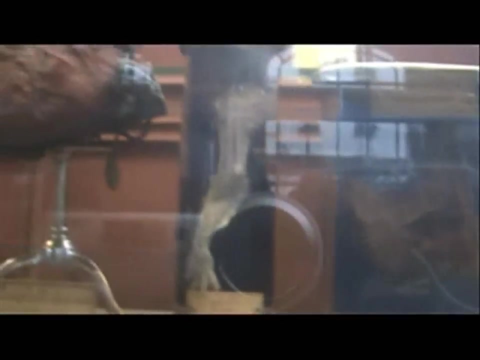 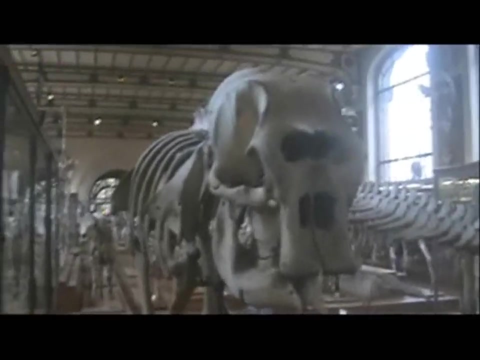 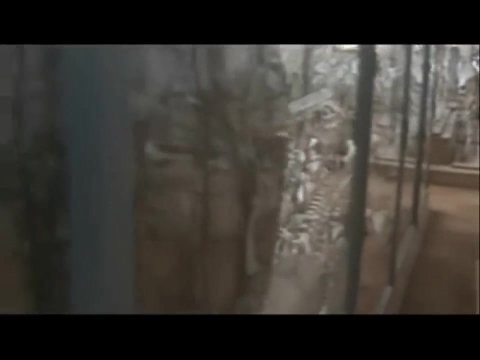 rhinoceros. oh no, oh no, sorry, we've gone from brains to like various body of the body parts. um so, people, this, they call this the museum of your nightmares in that fact article. but i just call it lunch. now we're getting to bigger skeletons. 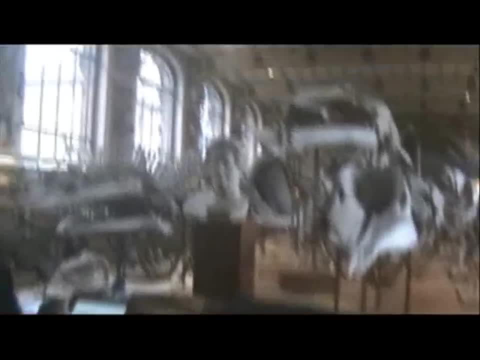 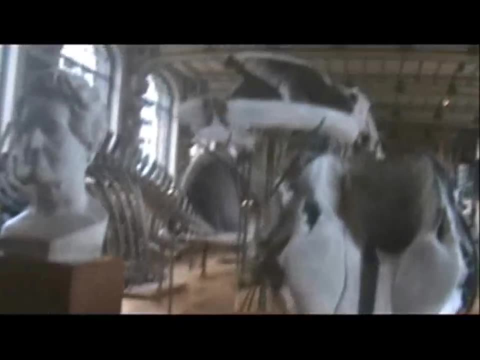 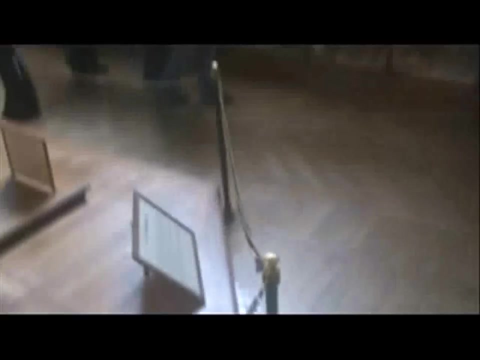 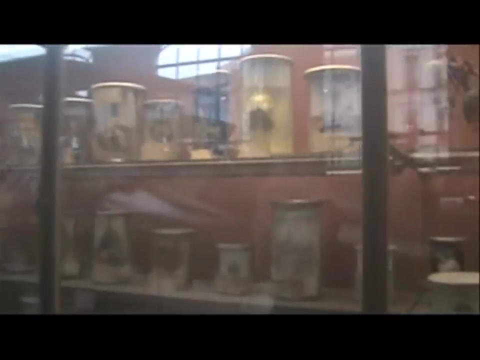 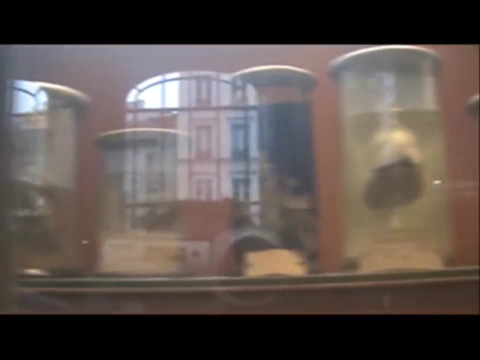 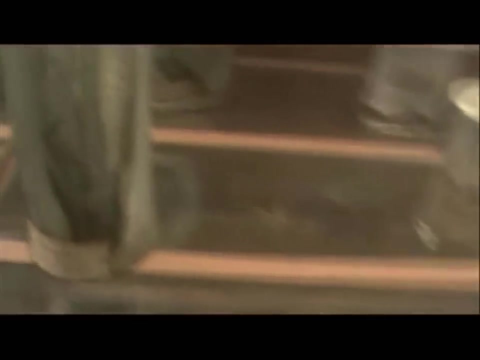 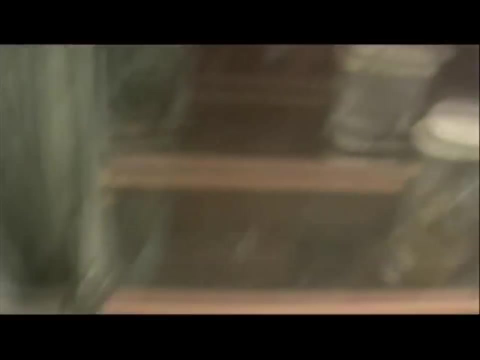 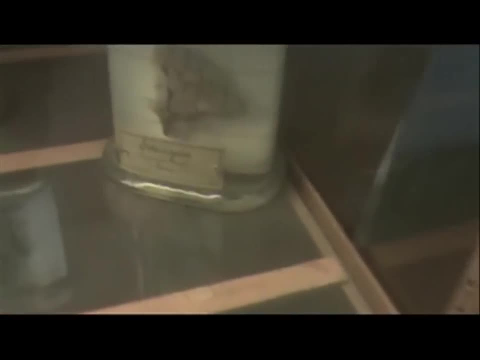 maybe i can like if i look at them on the internet, maybe i can break that stuff, but that's gonna be exciting. maybe i can like if i look at them on the internet, maybe i can break that stuff, but that's gonna be exciting. Let's see if I can figure out what they are. 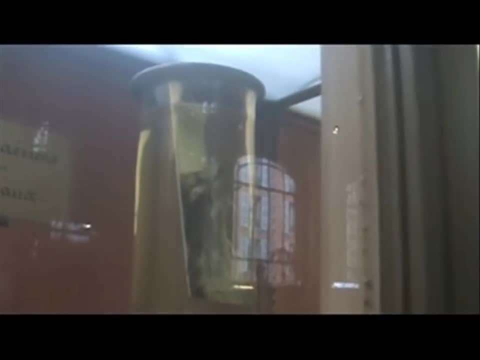 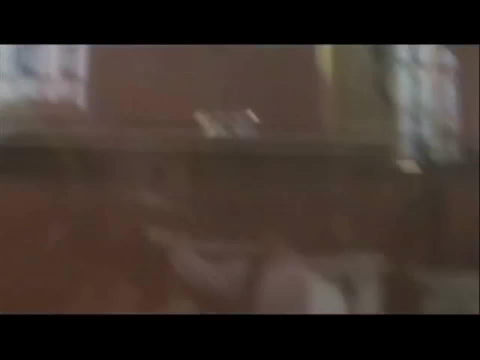 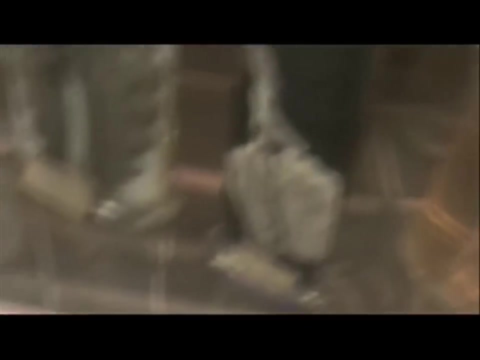 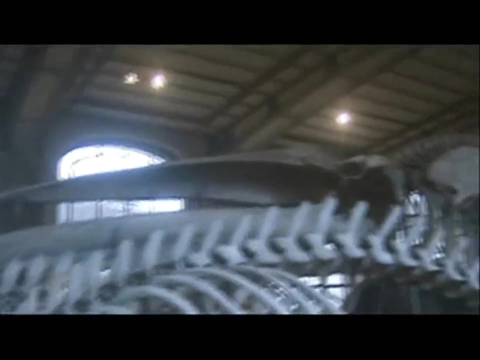 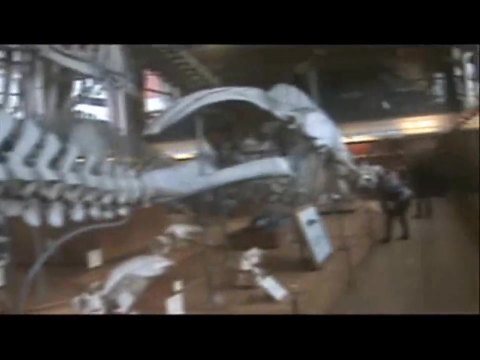 Ooh, It's a bird. Oh God, that's so sick. Lungs, Lungs. A boarded birdie. That must be one of the big whales, Little whales, Big ass whale, probably like a sperm whale or something. 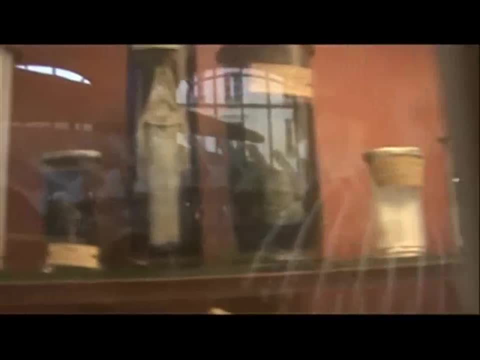 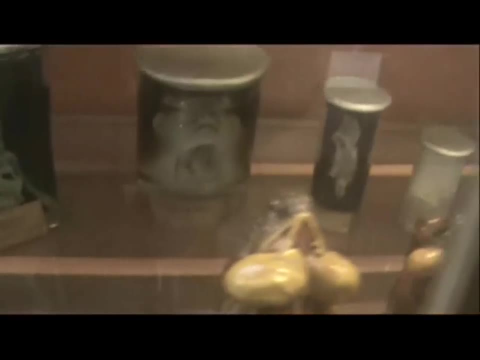 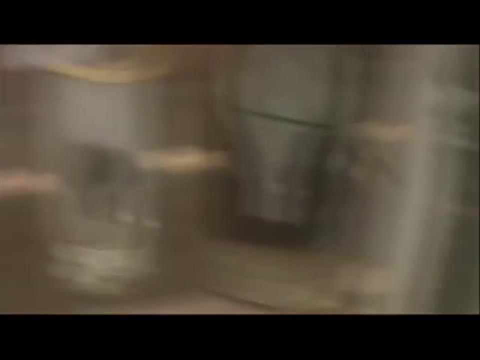 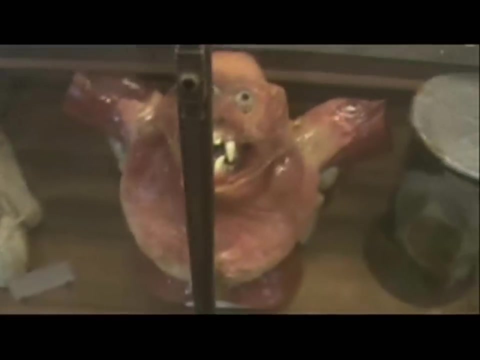 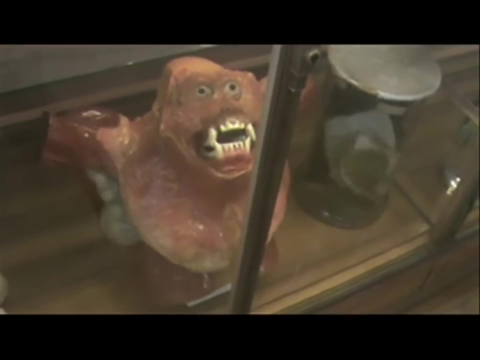 I'll come back. Crows- Oh my God, it's a monkey head. It's a monkey head. I've seen it before. Eh, a birdie monkey. Oh my God, Imagine waking up. you know what I wish I could bicycle like that. 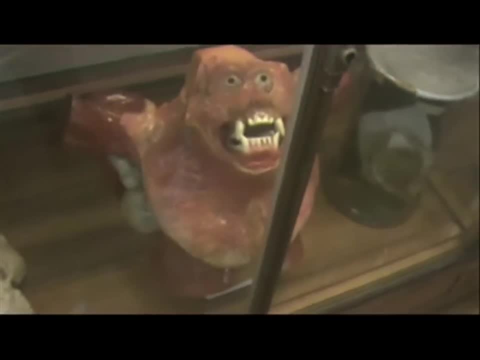 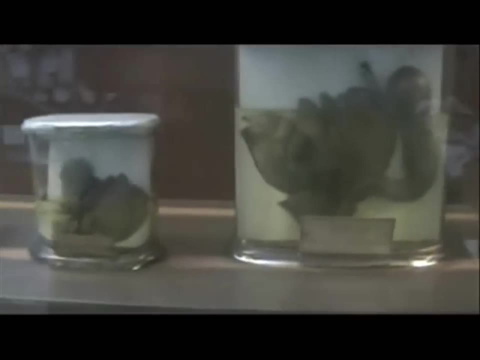 and then, like you know, when my roommate's sleeping, like sneak that in and so when he wakes up he sees that looking at him. that would be so scary for him, Funny for me, scary for him. Unfortunately, that wouldn't be fun. 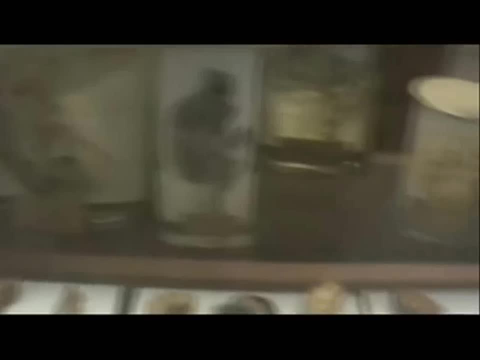 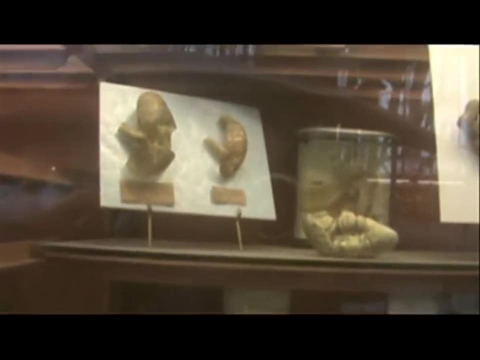 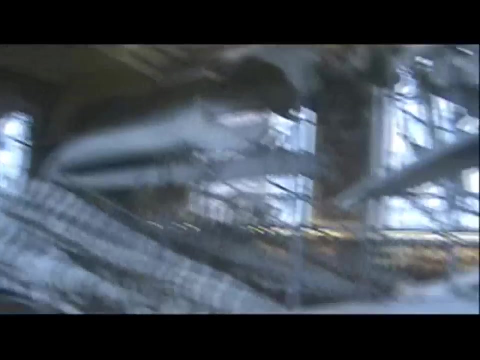 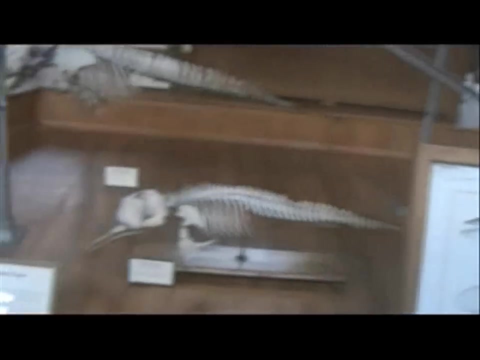 True, Look at that. I think that's maybe a sperm whale. I think this is a. yeah, I think that's a combat whale. This stuff probably like dolphins or something with theenga. Yeah, maybe, Yeah, a little bit. 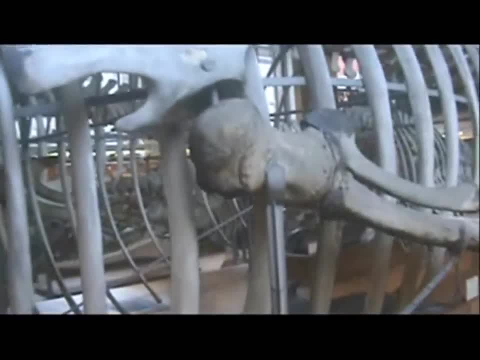 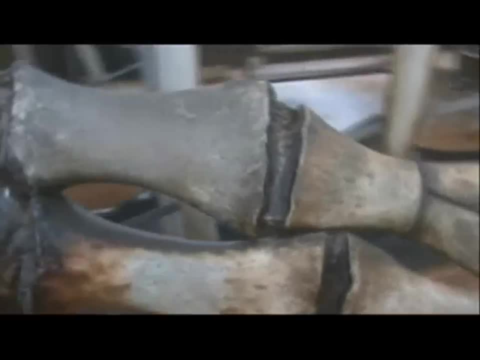 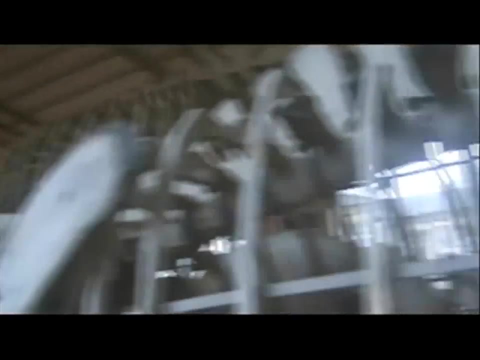 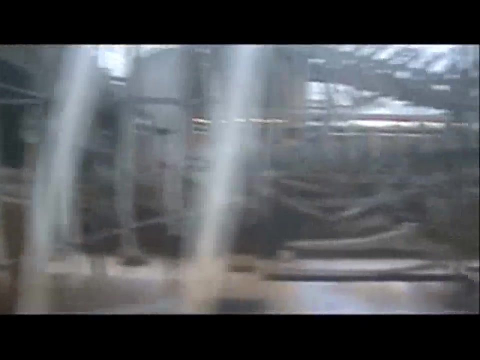 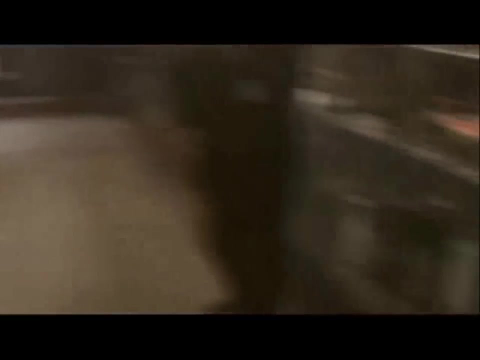 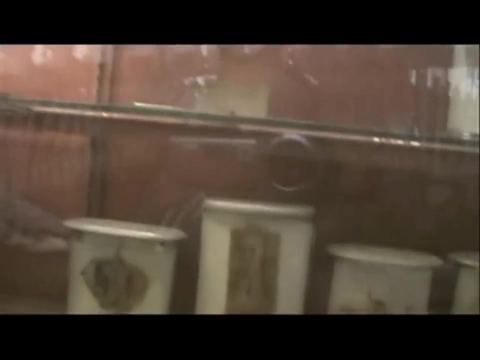 Oh my, there's a blue whale and then I think a sperm whale is over here and over there There's a blue whale, and then I think a sperm whale is over here and then I think a sperm whale is over here. 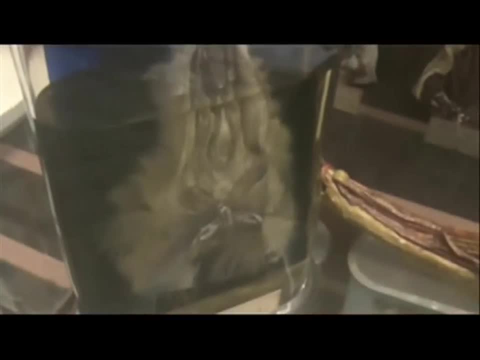 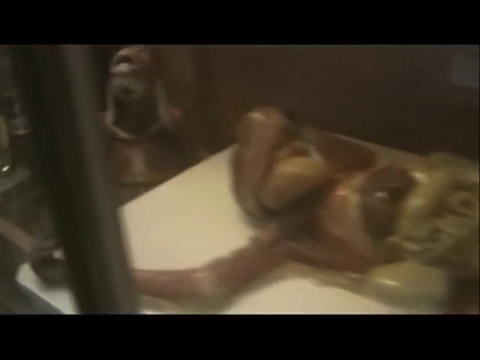 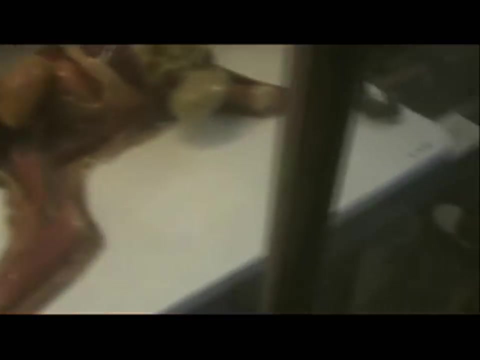 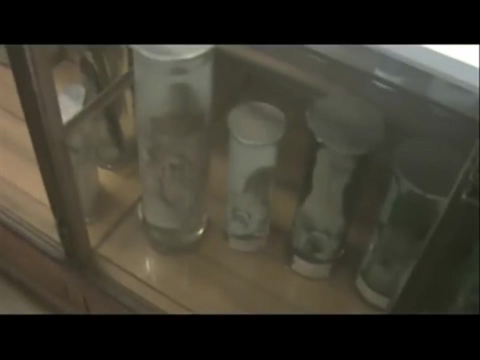 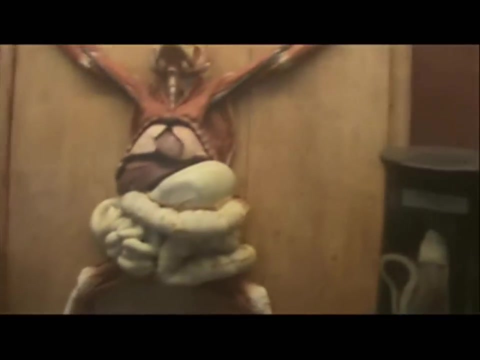 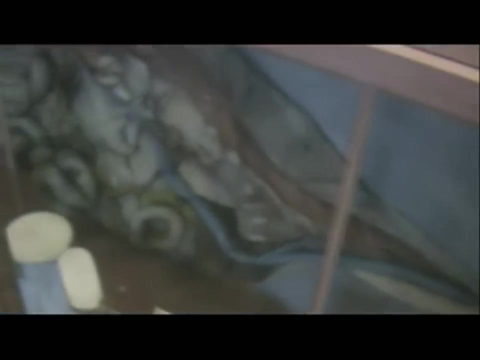 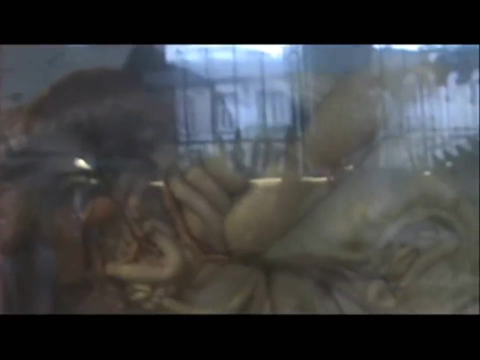 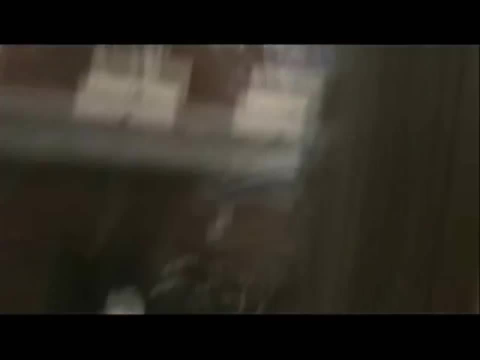 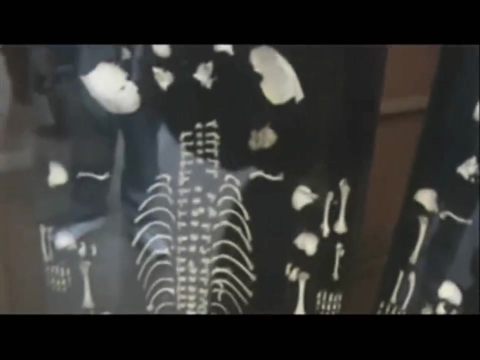 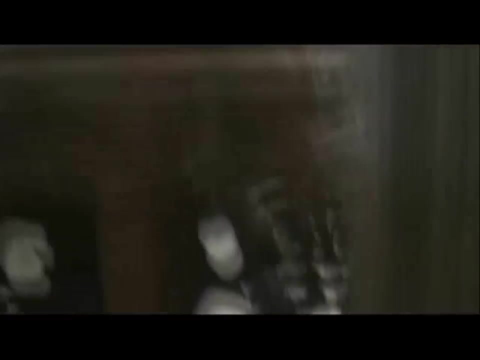 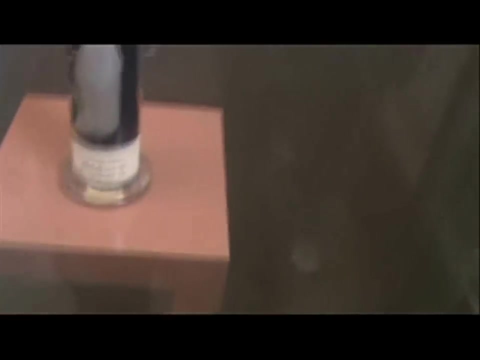 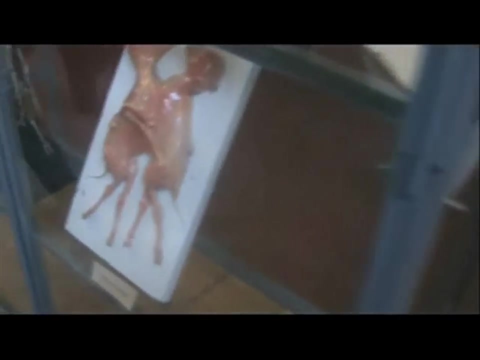 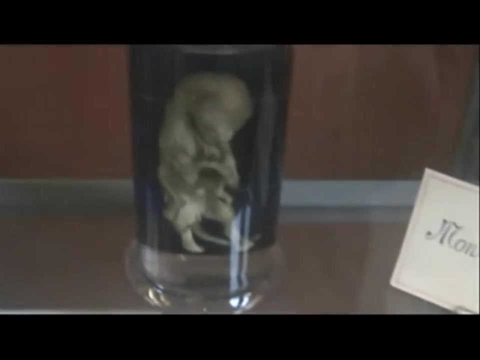 Little children, I think maybe monkeys, but they kind of look awfully like little mini humans. Wow, That's human Dead fetuses. Ah, that's nice to know Something from a dolphin. That's nice. Oh, There's a cat. 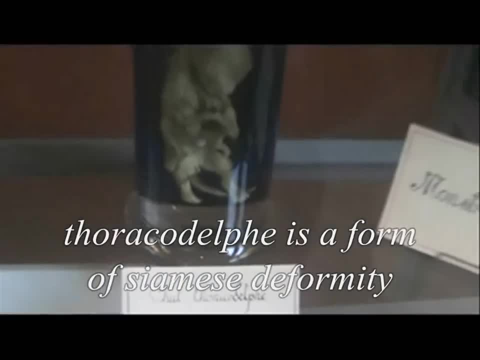 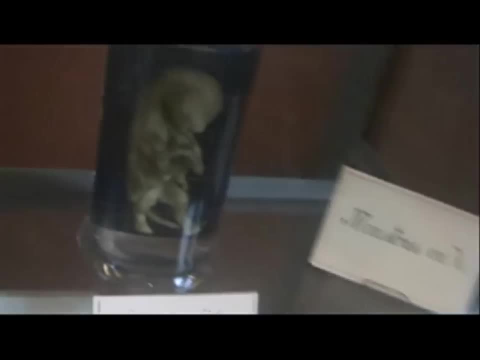 Because I know Cha is cat. Maybe it's like a tiger. It could be a tiger or something like that, but I'm assuming it's a cat. Looks like a little werewolf. Does that have like? Ugh gross, And there's a. 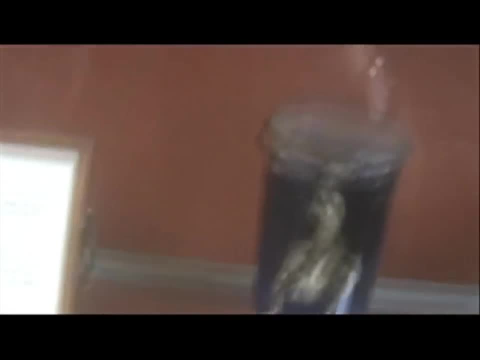 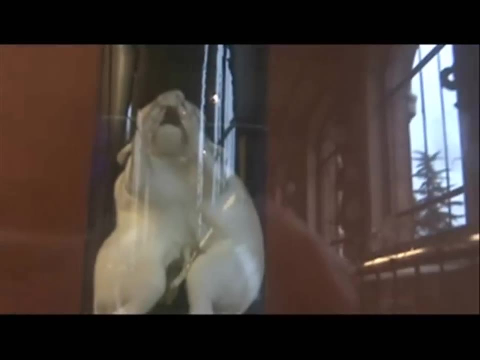 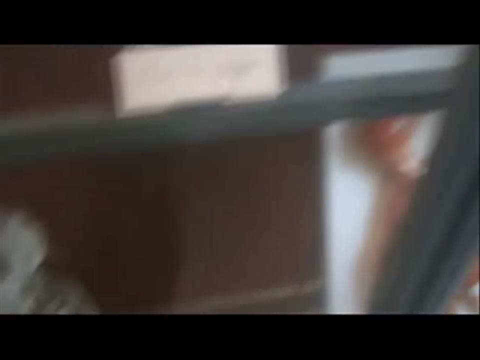 bird. Oh, these are like Siamese, I think. Look, These are like pigs, but there's like feet. that only looks like one head: That's a lamb. Yes, Yes, these are Siamese, Oh see. 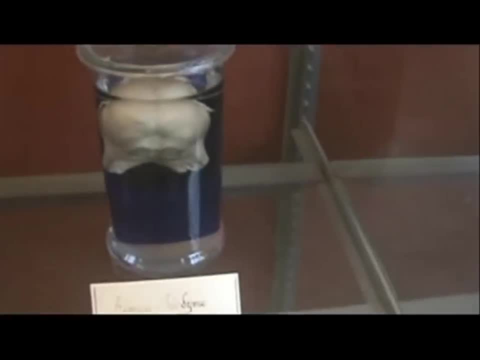 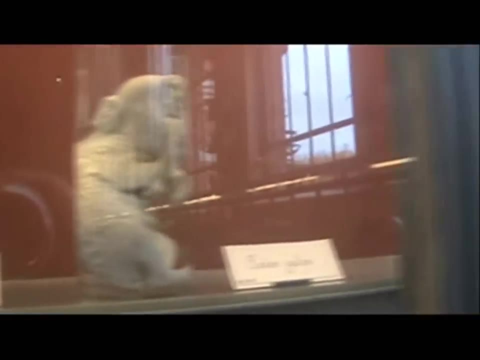 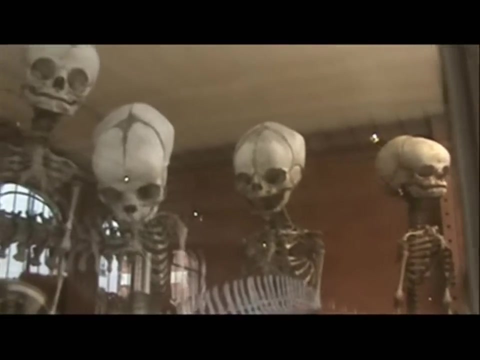 So they are like deformed animals: Two heads Monsters. I came back real. I came back real quick just to get some more pictures. and look at this one: He's a happy dead baby. Look at him, He's smiling. 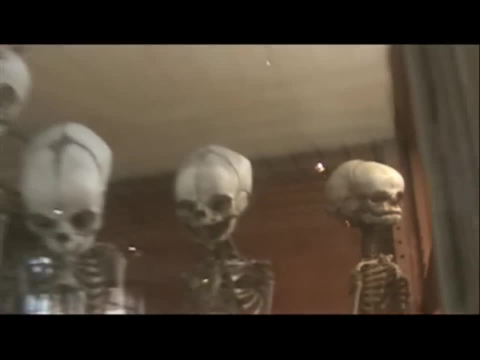 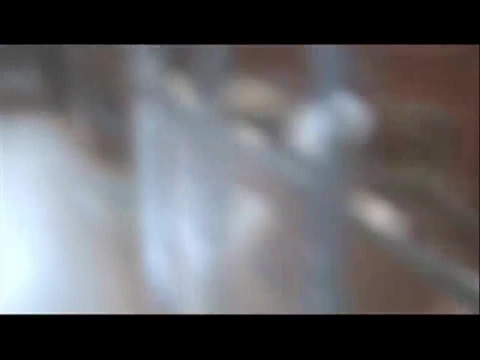 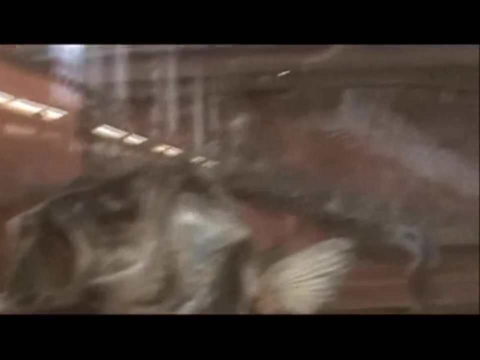 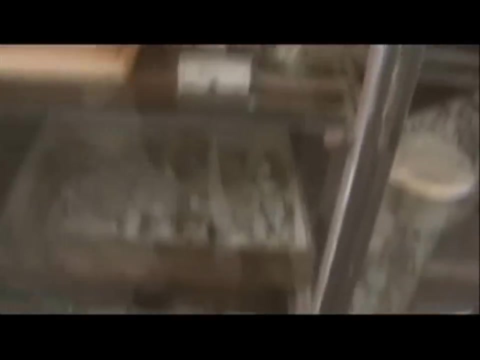 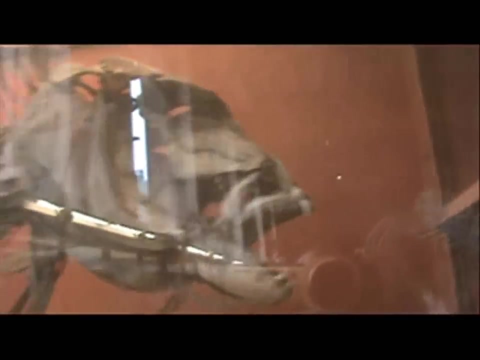 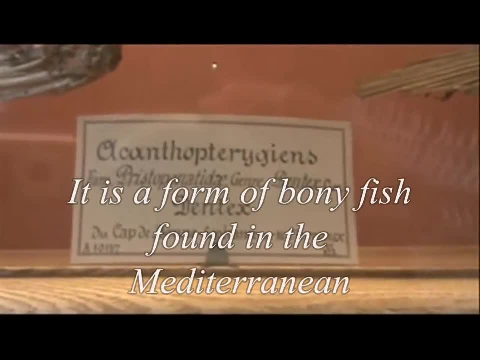 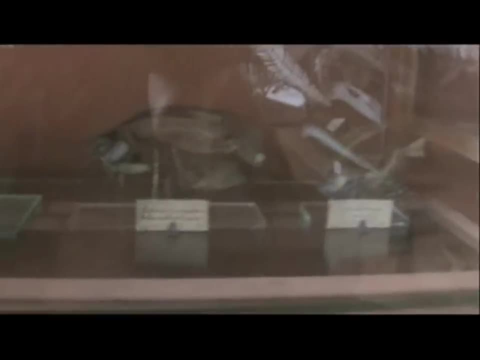 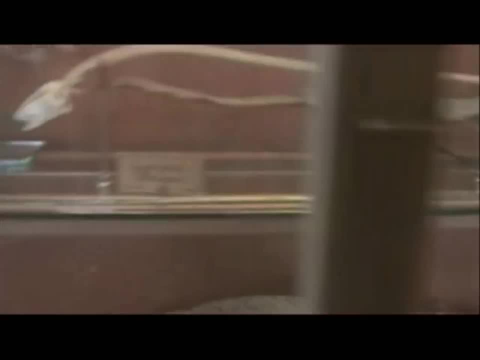 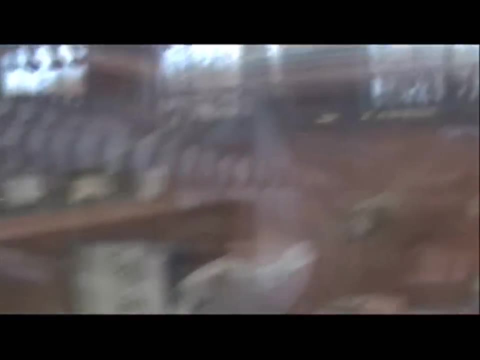 I think that's an eel. Yeah, yeah, I'm guessing that's an eel Electric eel. I'm guessing that's an eel Electric eel. I don't know what the hell that one is. I don't know what the hell that one is. 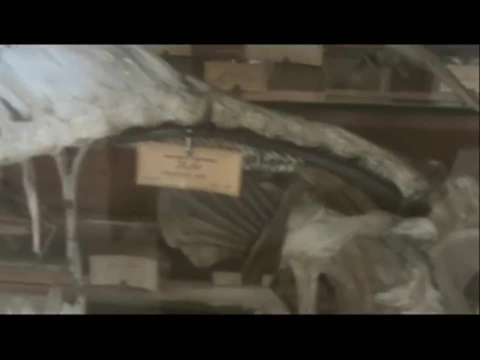 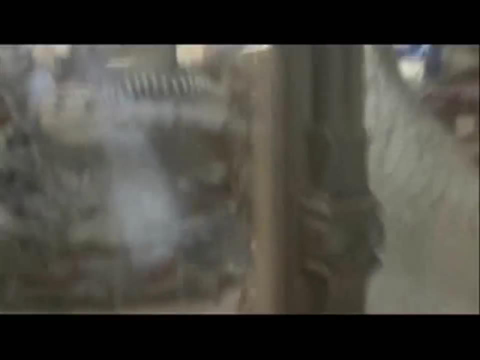 I don't know what the hell. that one is Kind of looks like an oversized angelfish, Kind of looks like an oversized angelfish, And this one looks like um, And this one looks like um, Oh, stingray. 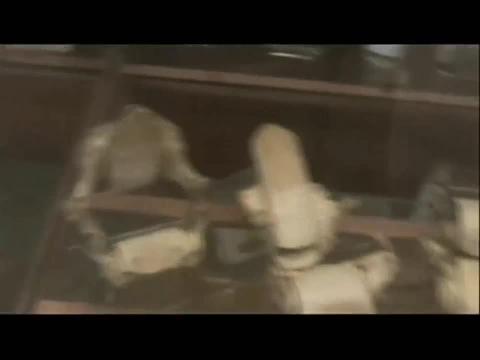 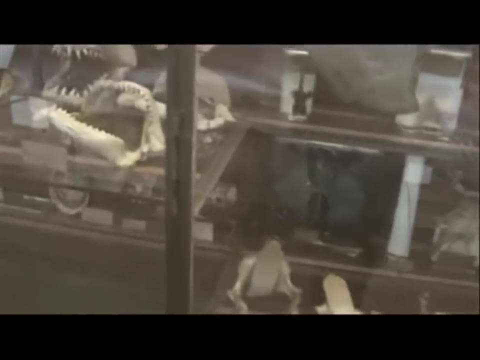 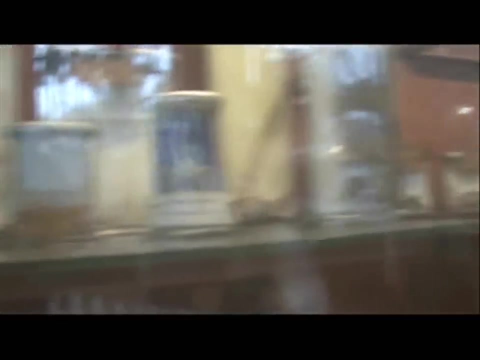 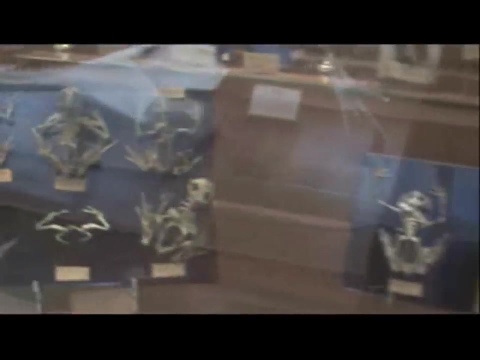 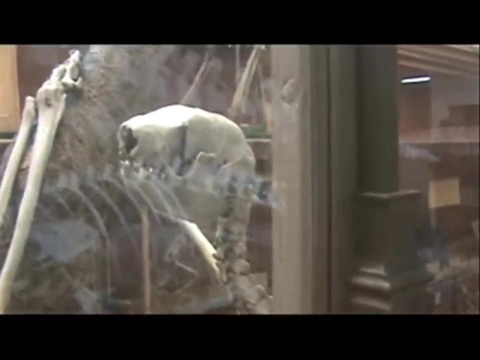 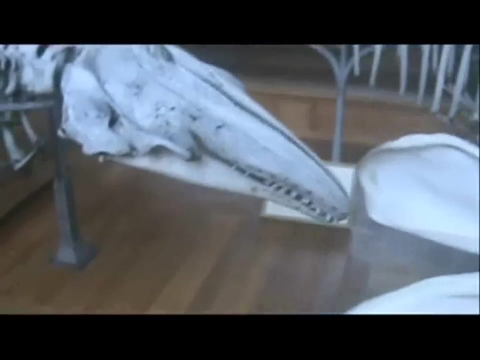 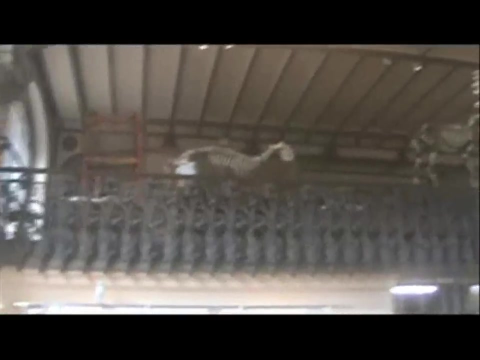 I'm guessing, Or demon from hell One or the other, Hammer Head, shark Head shark, Frogs, Frogs. There's some more stuff. I don't think that area is open, but I don't think that area is open but 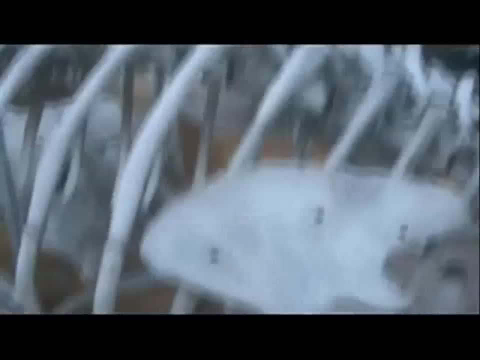 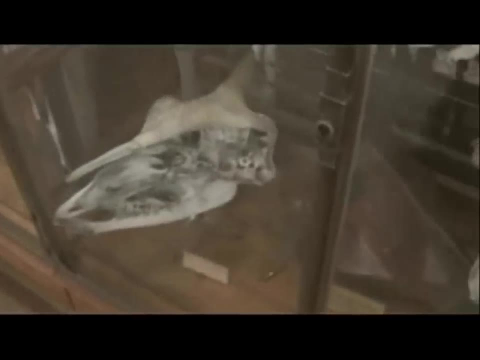 I am so glad I found this place. I am so glad I found this place. Thankyoucrackcom for bringing me to the land of my nightmares. You know, it wouldn't be so bad if we didn't have these creepy little skulls. 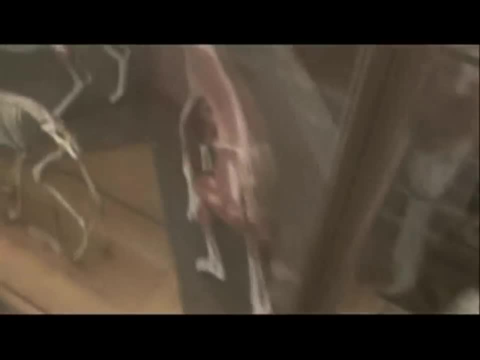 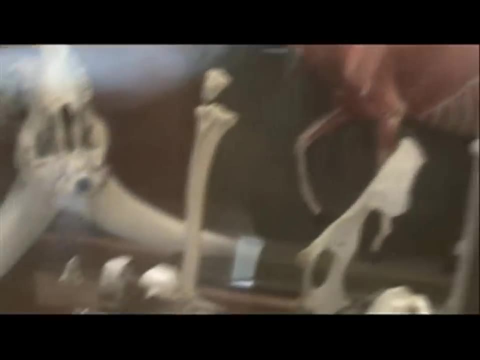 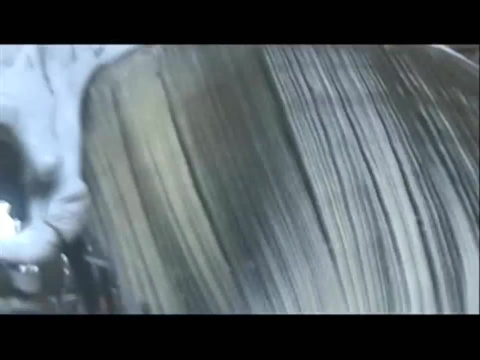 if we didn't have these creepy little skulls and stuff like that. Nightmares is like howries or ripped apart animals, like there's a goat- Oh see, they're sane. Oh see, they're sane. Oh, Oh my. 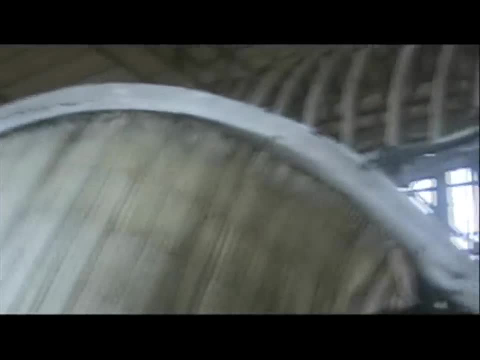 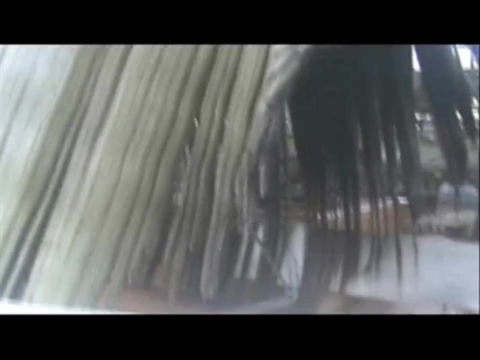 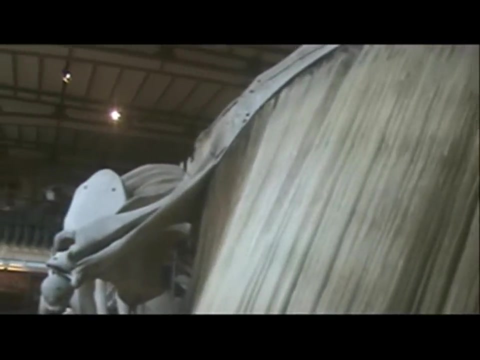 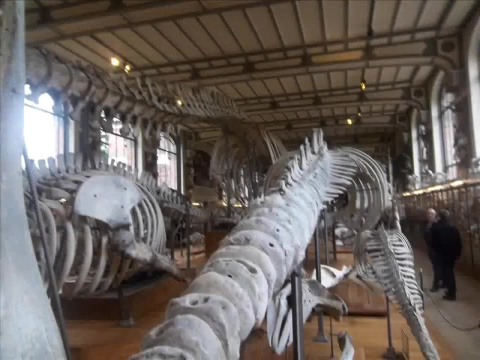 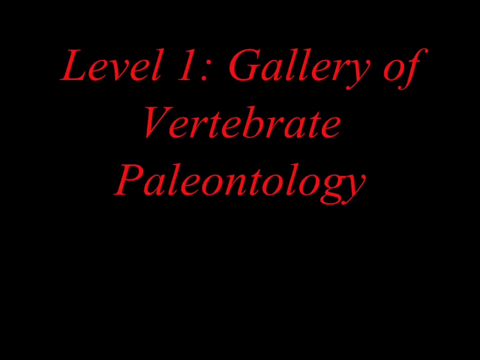 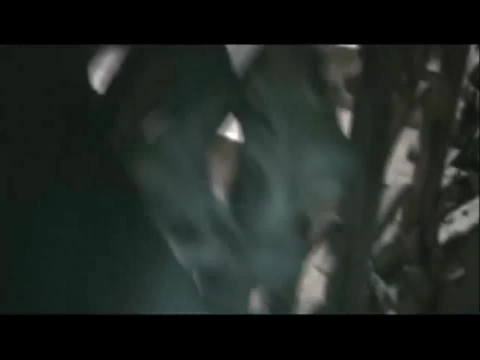 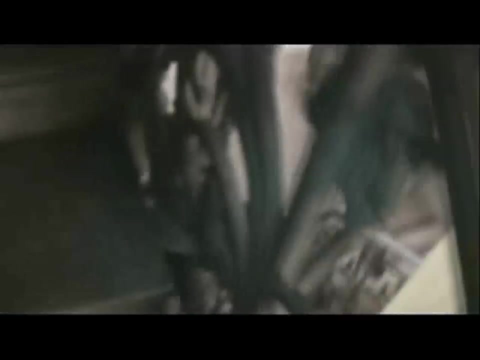 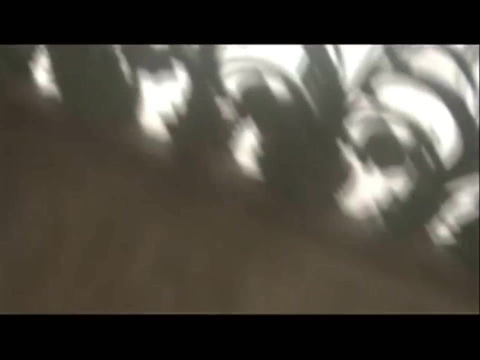 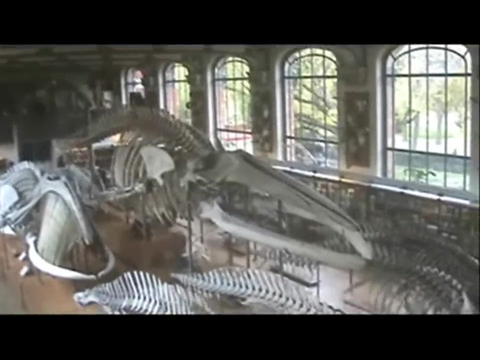 So I'm going to the second floor now. Get the IR lights on now so I can use it, You know, to get better at this stuff. Oh, yeah, Oh, you're going to the front, Yeah, Yeah, OK. Moment of silence. 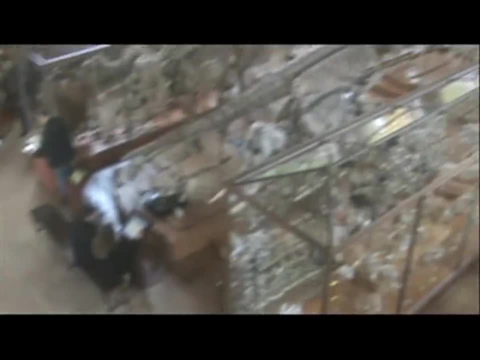 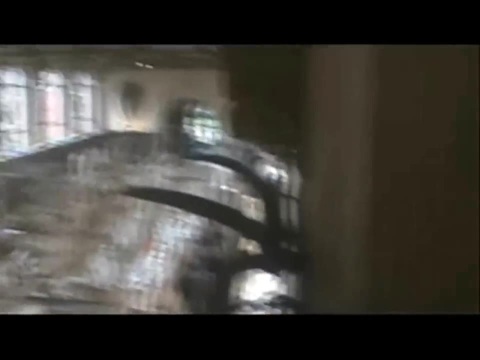 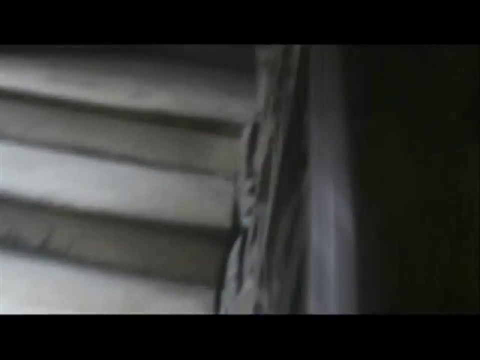 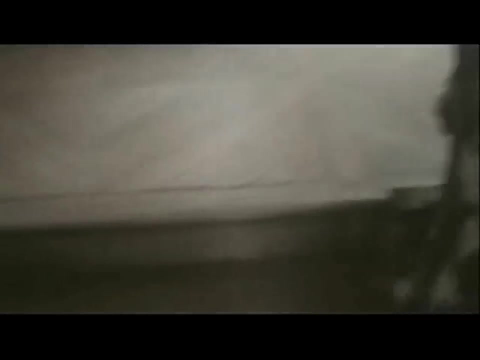 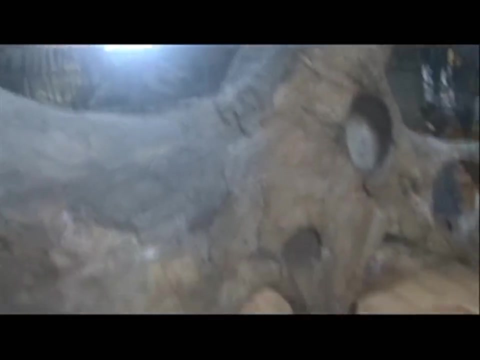 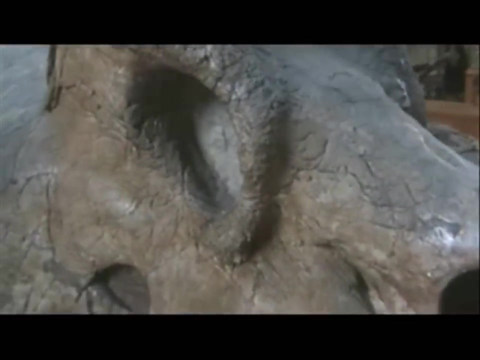 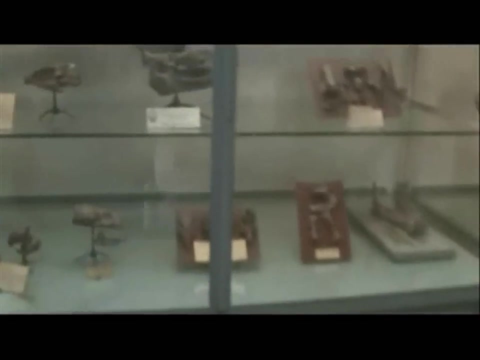 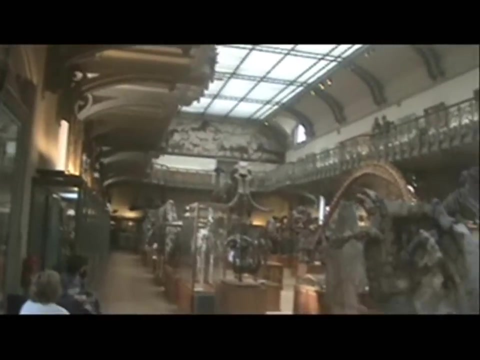 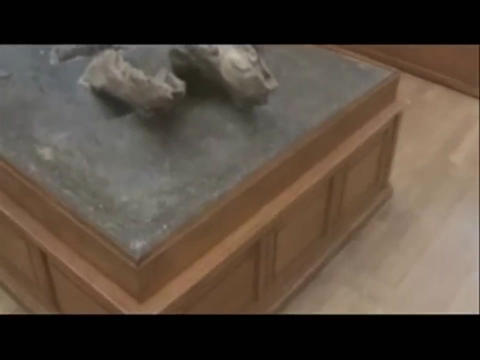 for the dead. OK, Moment of silence for the dead. Ah, Yeah, Yeah, Ah. Let's see, you can imagine what the second floor has in store. Well, now we got long dead creatures, dinosaurs, in body parts. Hello. 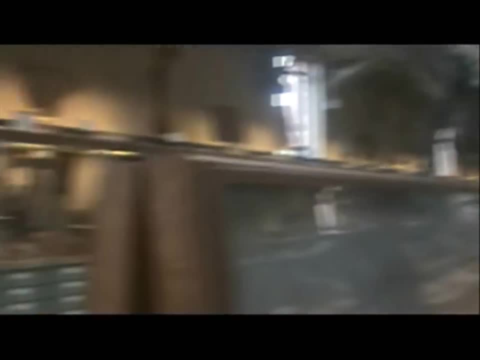 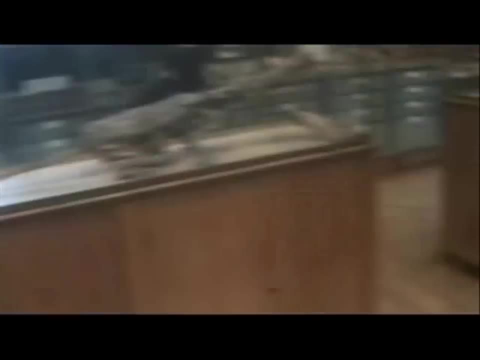 Look at that teeth. This is one of the few museums where you can actually really get up close and personal with some of these fossils. And it's a Tyrannosaurus Rex, I do believe it is. I think, Yeah, kind of judging from the head. 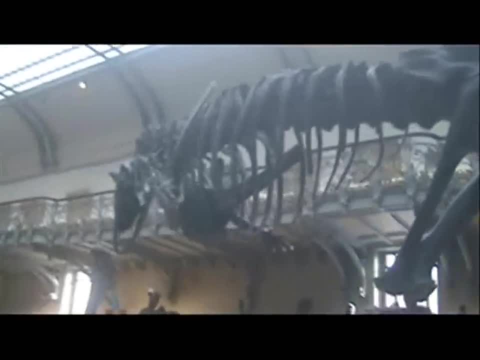 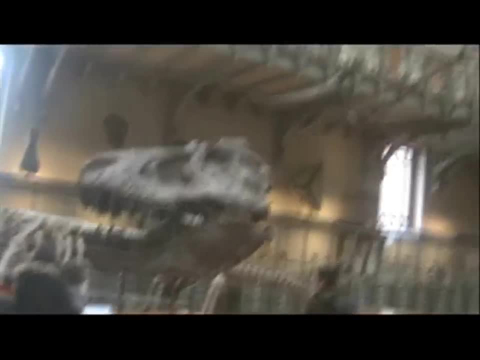 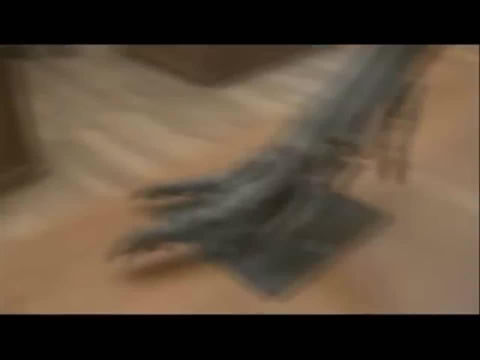 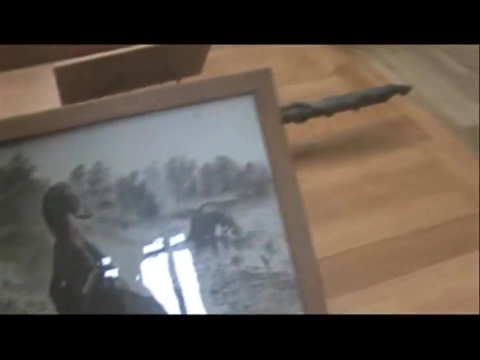 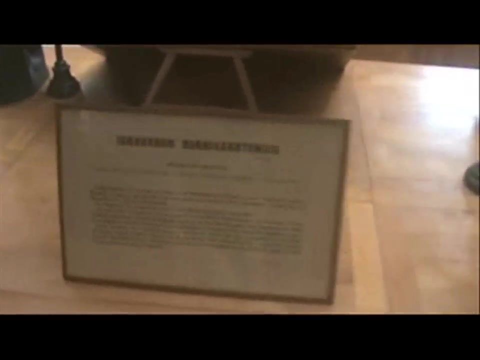 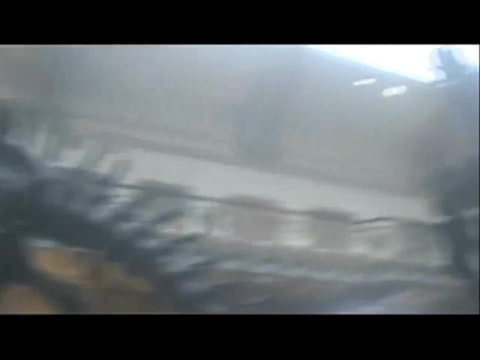 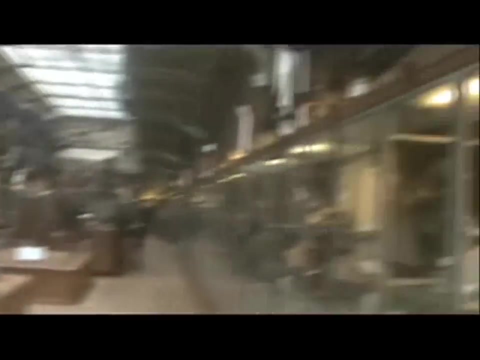 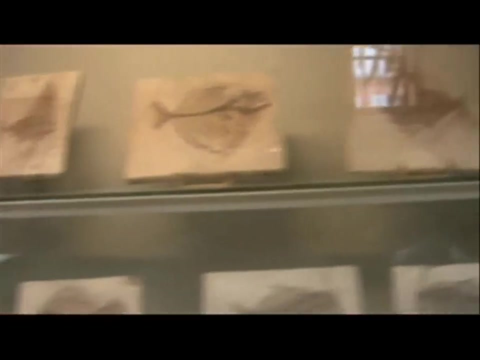 Don't know what that is, But I think that's a T-Rex. But I know what that is: Iguana Don Apatosaurus over there, Iguana Don Iguana Don, And this is not so creepy, just, you know, just regular fossils, but I mean the downstairs. 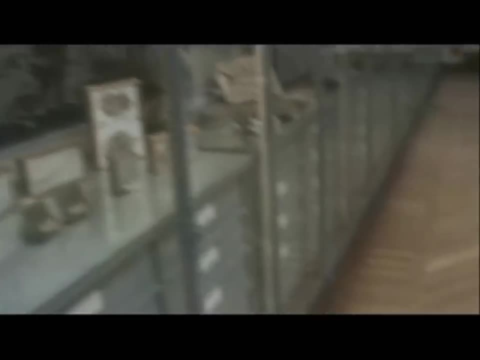 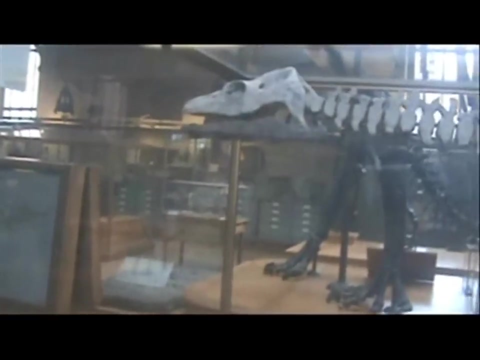 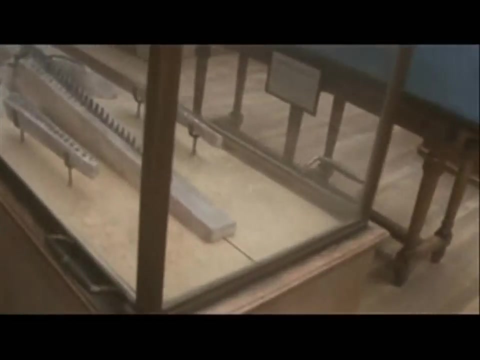 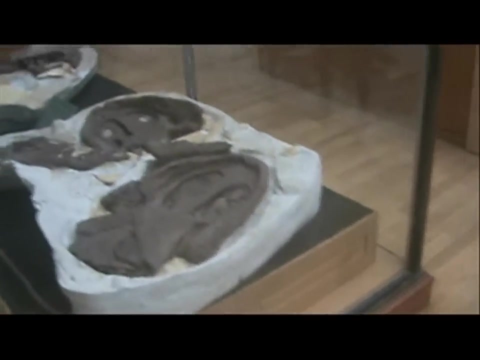 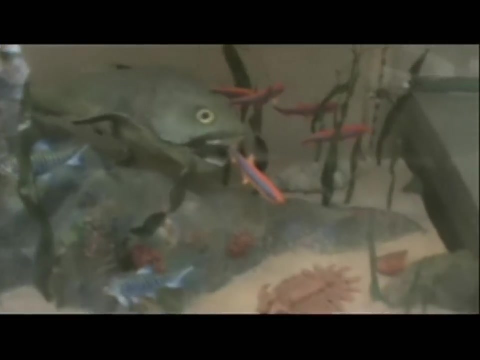 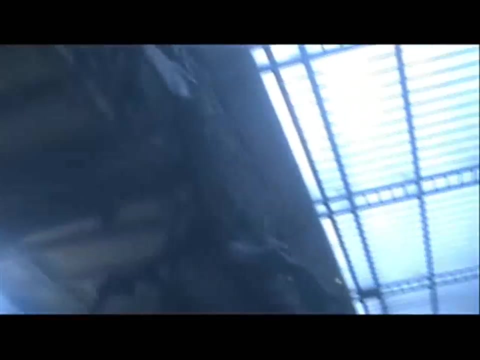 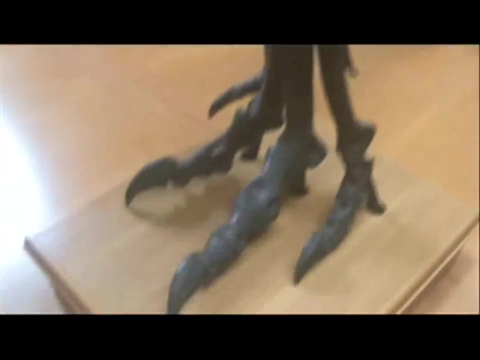 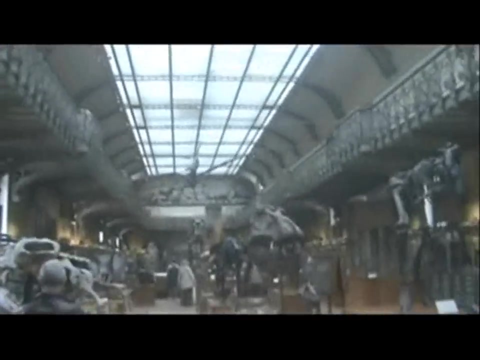 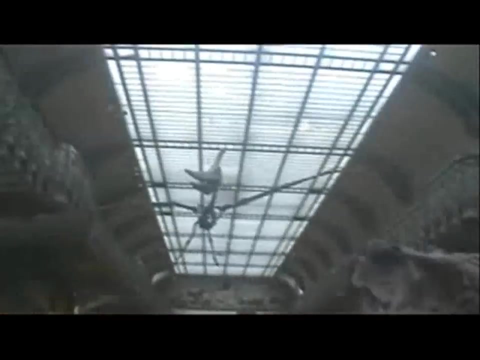 was creepy with all the bodies and formaldehyde and everything. This is just fossils that I'm going to show you anyway. Oh, now that's awesome. Welcome still in Dinoland. Got to go more down here too. Pterodactyl. 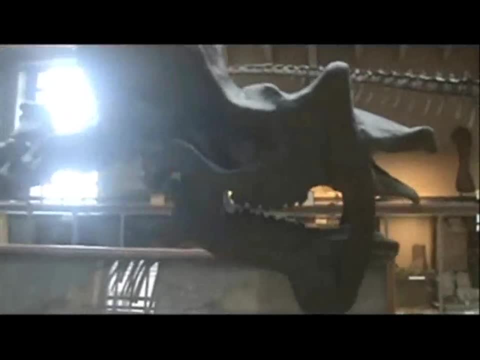 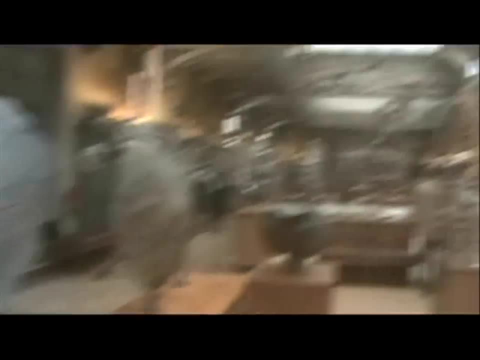 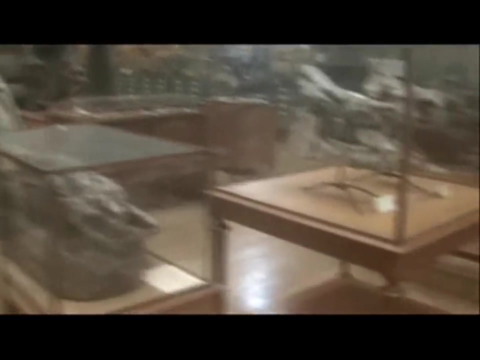 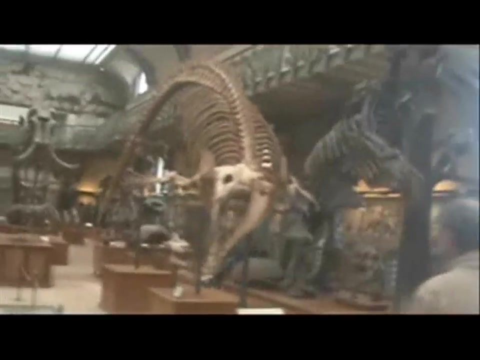 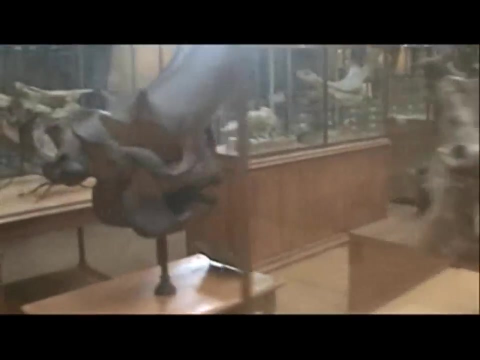 Pterodactyl. Pterodactyl One, two, three. Welcome to Disneyland of Tinian Island. Welcome to Dinoland. Welcome to Dinoland. Welcome, Welcome to Dinoland. few artists around here. I can see why. you know they come here to draw some of. 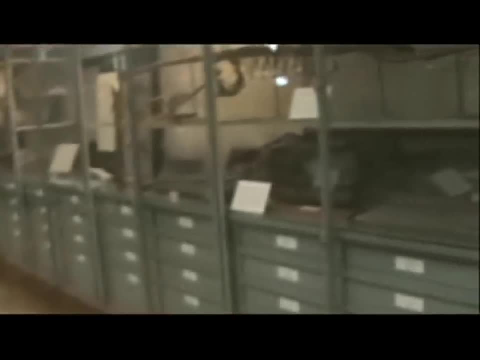 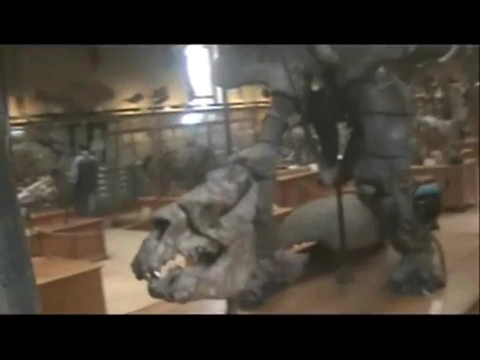 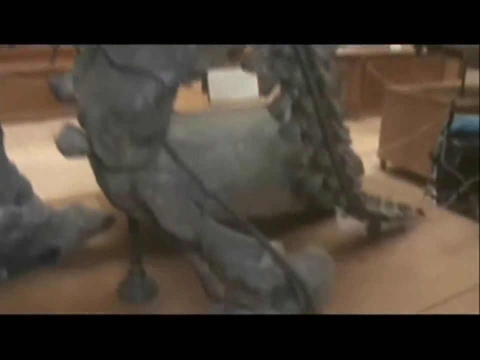 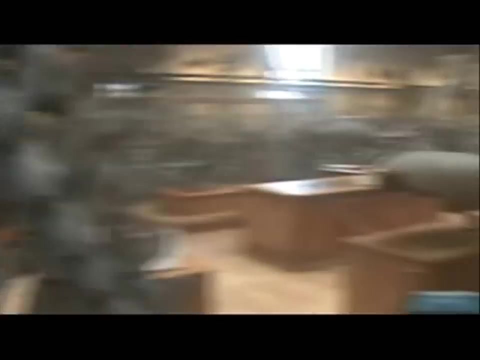 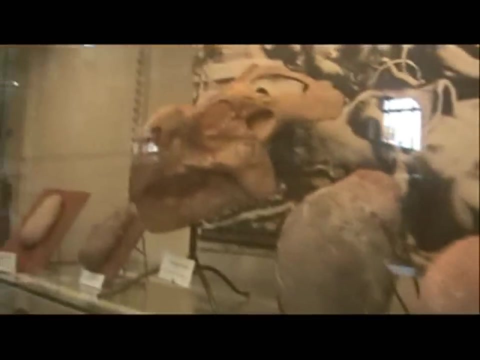 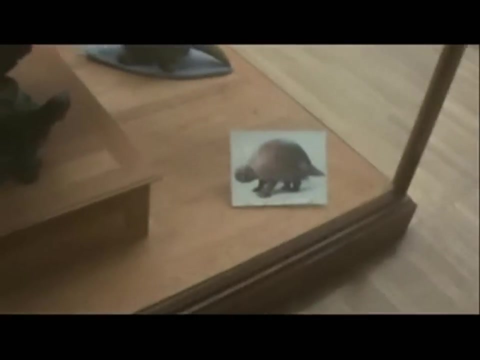 these skeletons. it probably helps fine-tune details and their skills, but these suckers are big, aren't they? these must be. I think these are ice age creatures, because I know down there that must be the wooly mammoths you, and that's what that looked like. 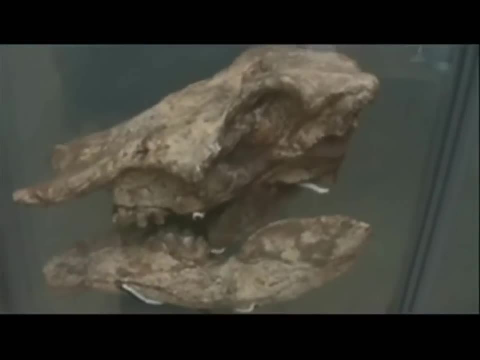 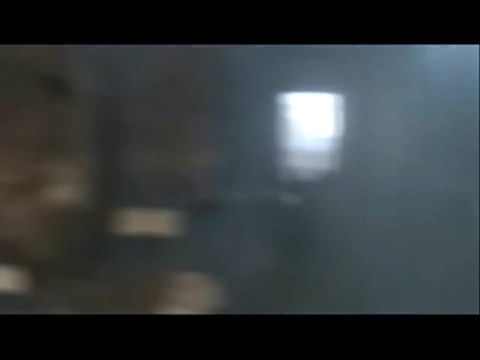 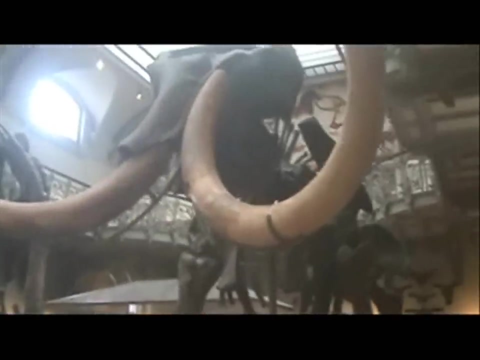 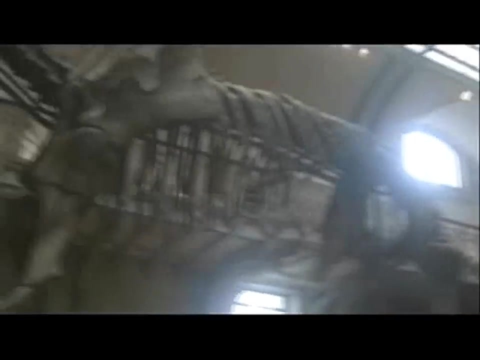 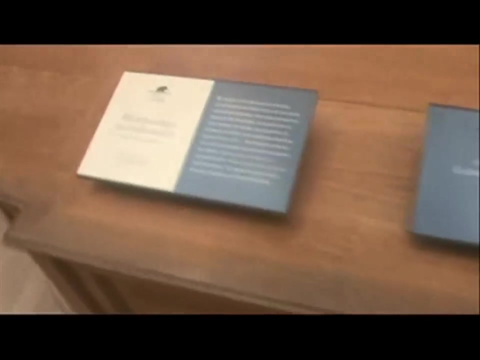 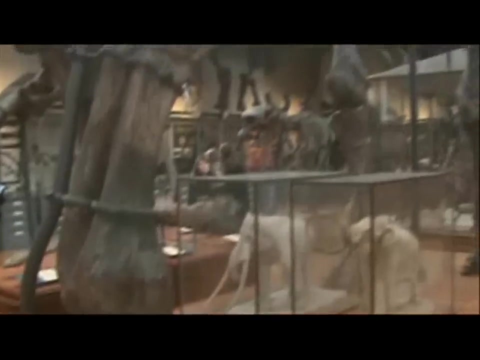 origins of evolution of the elephants. hey, I got it see: origins of evolution of elephants, which I'm assuming is what it means somewhat, since we're near wooly mammoths and stuff like that. oh my god, these sick suckers up close and personal. maybe that's a wooly mammoth and that's an elephant, I don't know. I don't think so. I 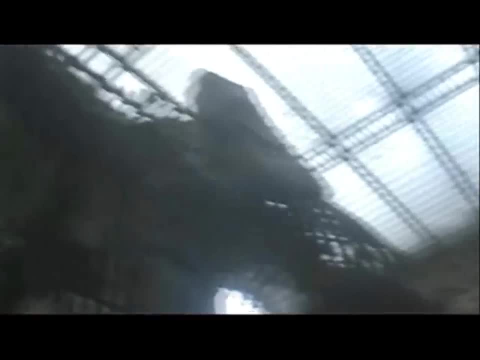 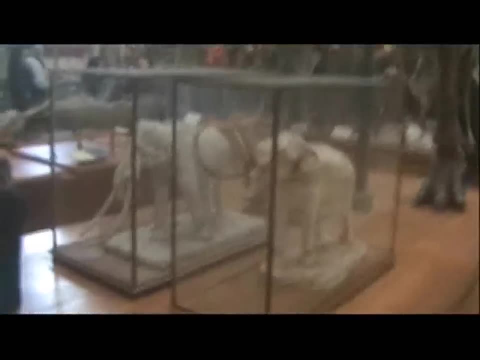 think that's a wooly mammoth and that's an elephant. I don't know. I don't know. I didn't know elephants were that big and maybe their ancestors were. yeah, it must be like ancient elephants, even though that looks quite like an elephant that I know. 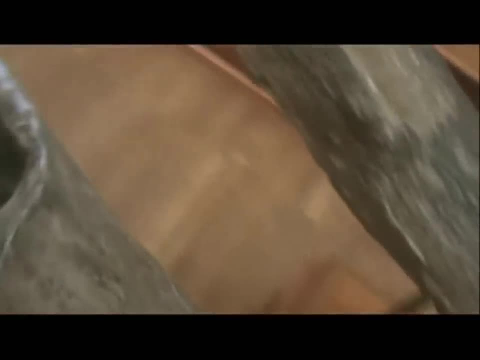 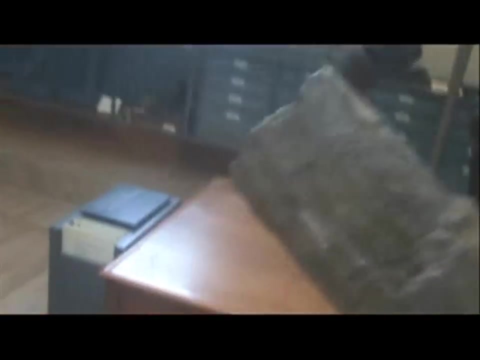 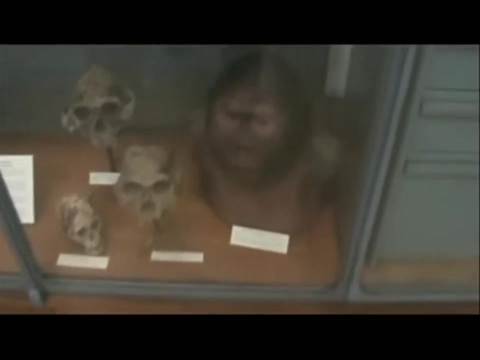 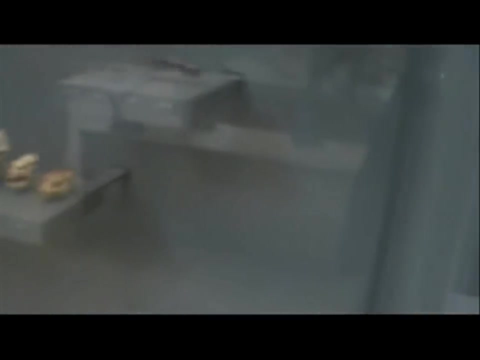 oh, yeah, that's a good one. this is going to be a little lucky. yeah, this one's a little bit more difficult, but it's a good one. yeah, cool, maybe we'll go with it. It must be Zira from Planet of the Apes. They show details here. 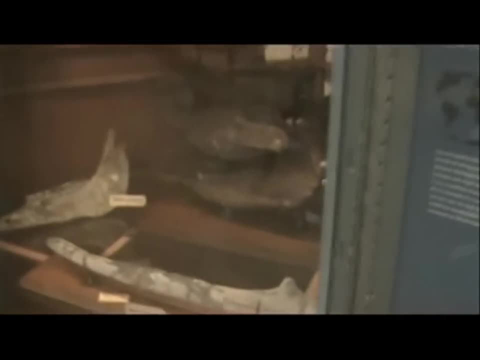 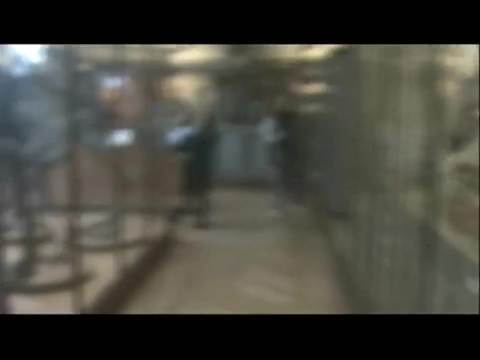 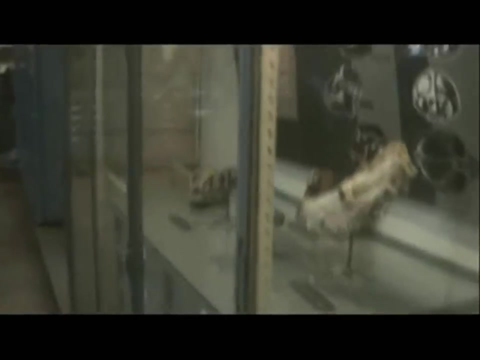 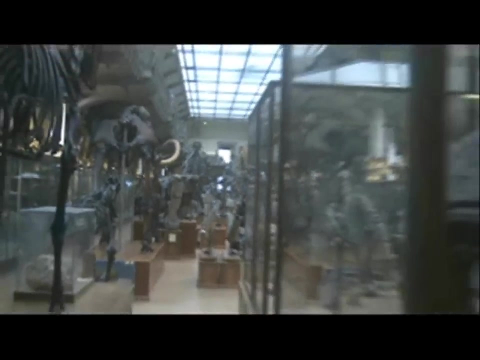 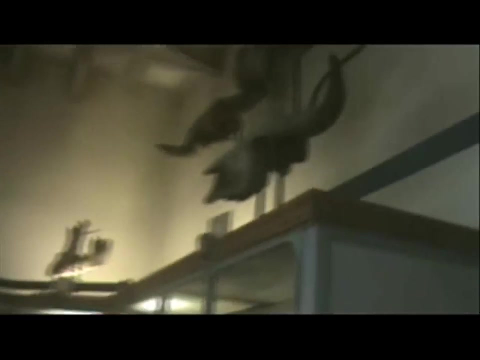 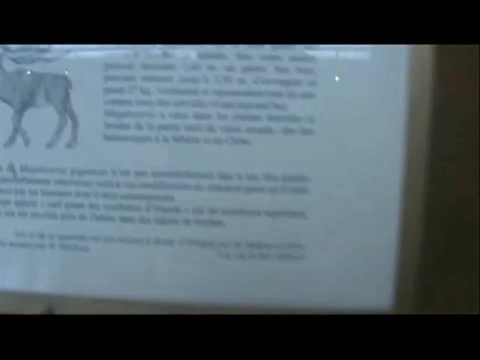 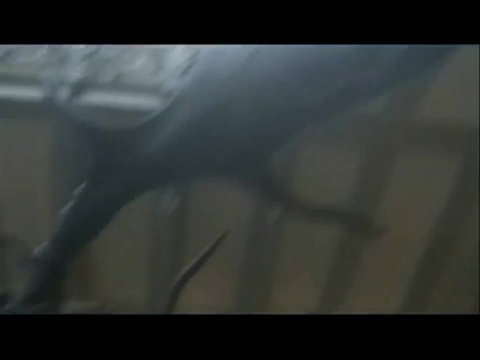 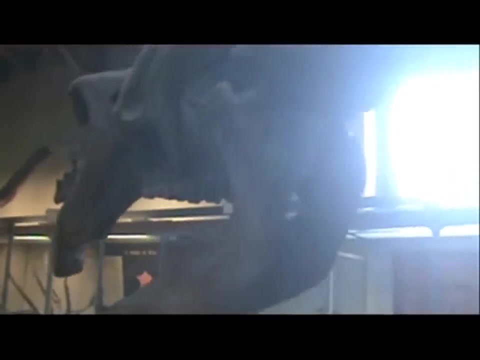 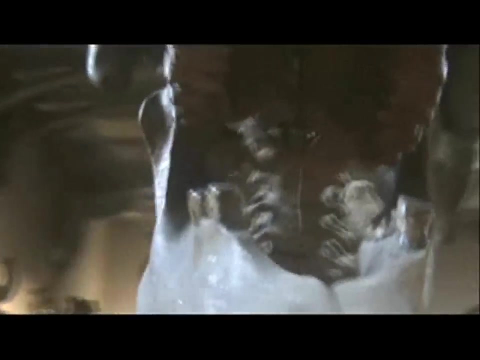 Wow, this is a really cool place. I think it's still appropriate for creepy places below, even though there's going to be no ghost, No explorations or anything. Elk or caribou, Ancient caribou, Elk stuff. Alright, maybe I should go to the third floor anyway. 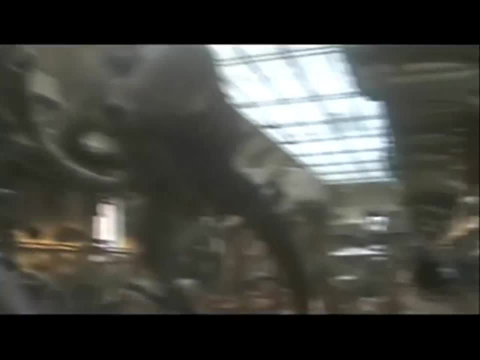 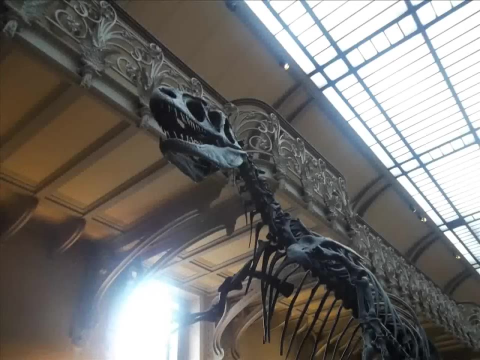 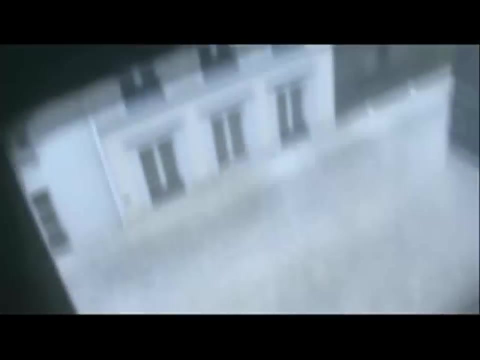 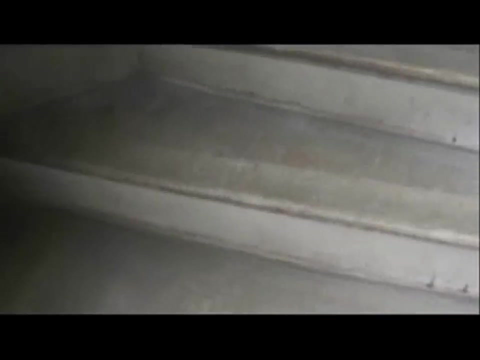 Alright to the third floor. I made it to the third floor. It's a very old building, that's for sure. Here's Paris. I still haven't gone to the Eiffel Tower yet. Maybe I'll do the opener for this video in front of the Eiffel Tower. 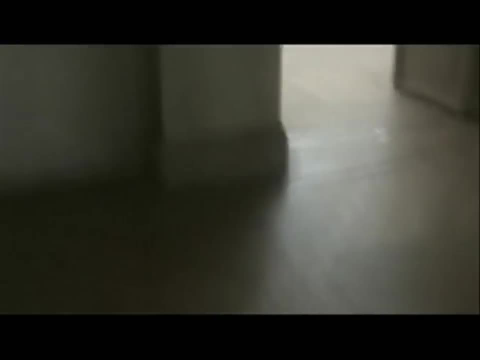 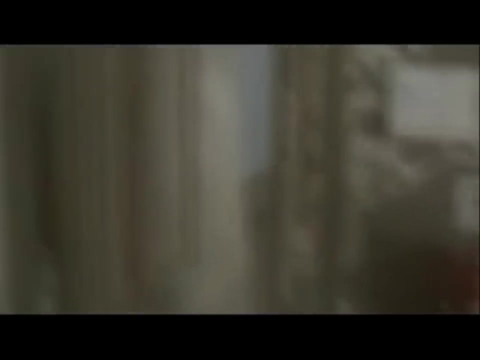 Yeah, yeah, I have been to the Arc de Triomphe and Notre Dame already, which is also made into a video. Here we are, Heaven. I wonder what that means. Oh, Now we've got seashells, Rocks. 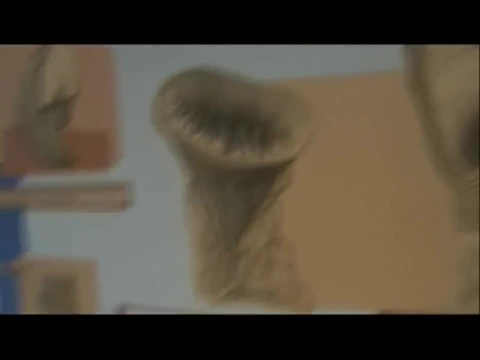 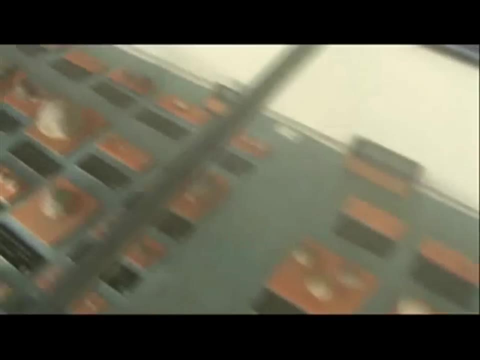 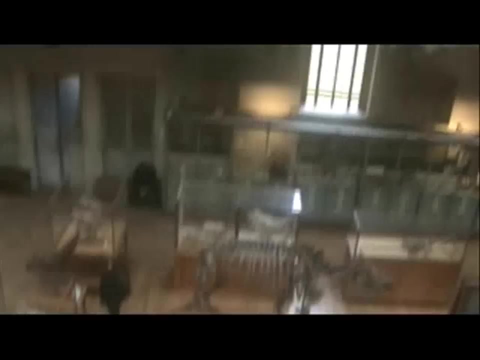 And more shells. HP Lovecraft must have came here. Looks kind of like something from his dreams. Not as impressive, I think they're mostly like seashells. but I'm going to go around anyway. But here's a view from above. 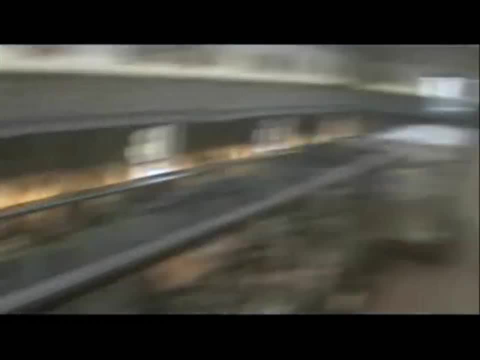 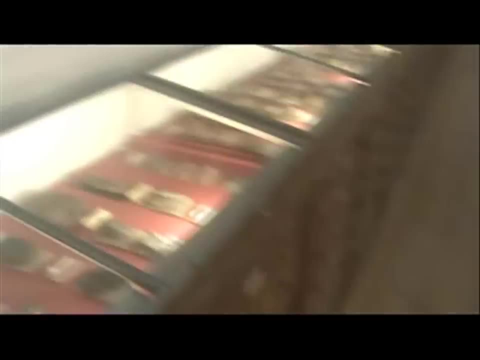 I'm going to head down this way, go around and then probably head back downstairs. Um, I think I'll end up leaving. Wow, It's just so cool. I don't know French, so I'm not reading everything, I'm just looking at everything. 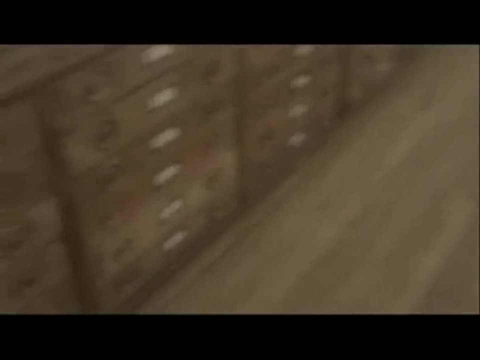 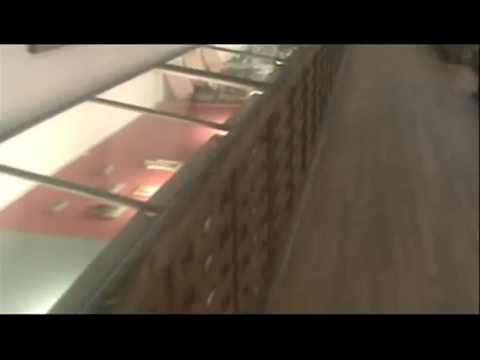 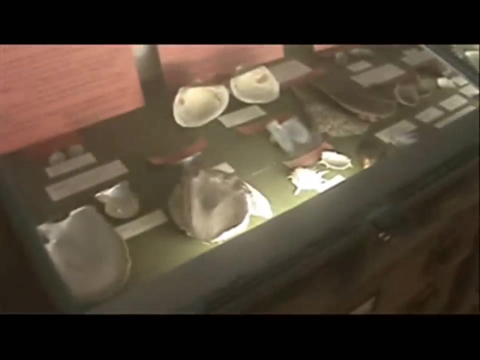 Except for like the few words that I do know and that's not enough to like really go through a museum. I guess one came to the whole crack article. Uh, I think the nightmare part is like the first level. 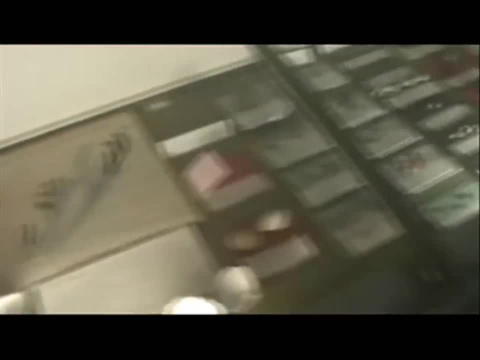 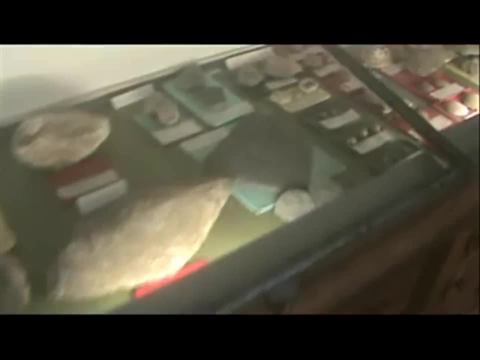 especially with all the like, the weird body parts and formaldehyde and the deformed animals and stuff like that. But up here it's just not bad at all. There's a statue that I got to show you out in the front. 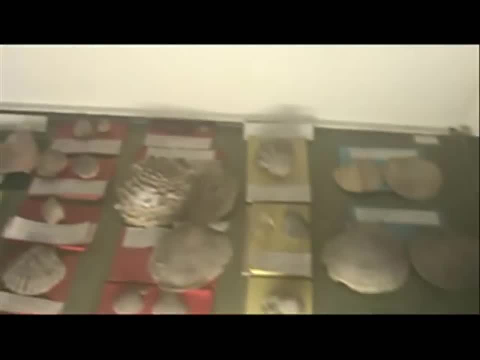 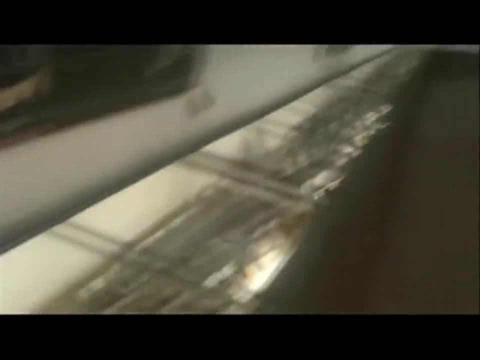 It's very creepy. You're going to love it. Yeah, this is more like seashells, Seashell, seashell by the seashore. It's like a little like old fresco, fresco, fresco painting. 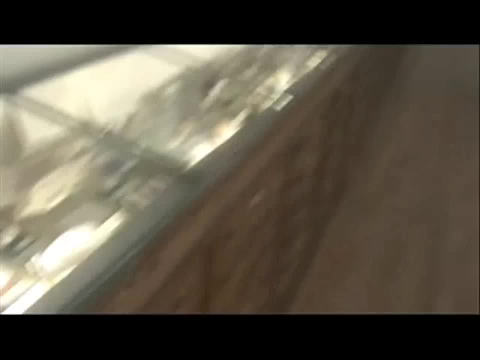 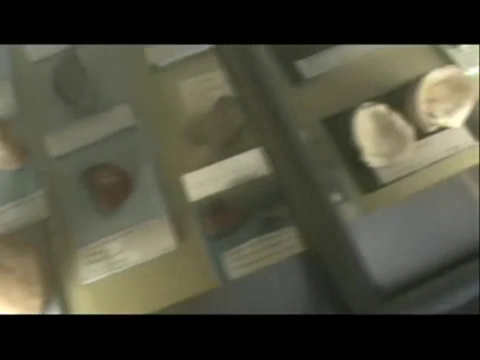 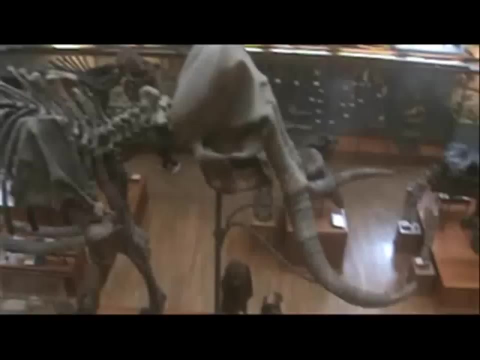 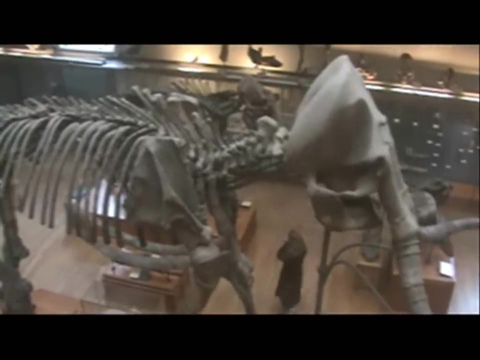 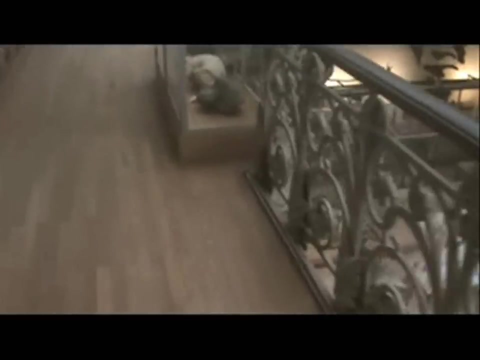 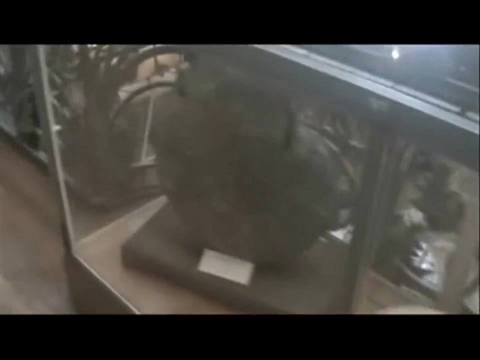 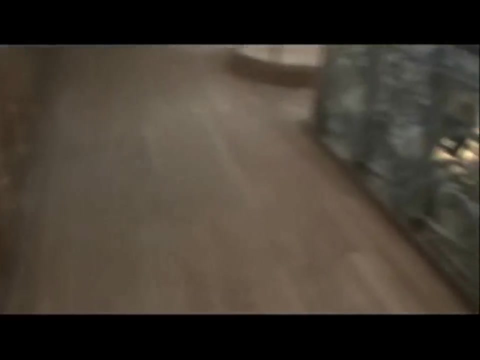 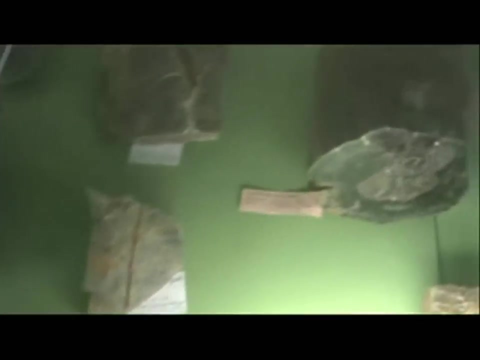 of like some old cave drawings- Pretty cool. This is a cool view of that uh elephant, woolly, mammoth, ancient elephant thing. We've got a full like lots of fossils And, like I said, this is just one part of this whole museum area. 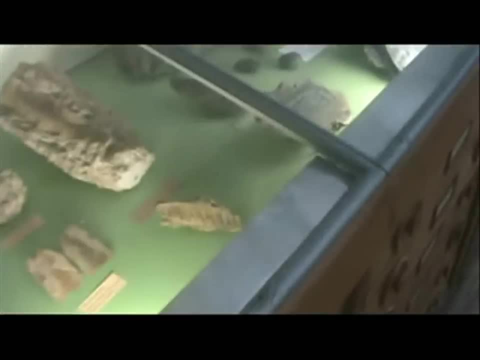 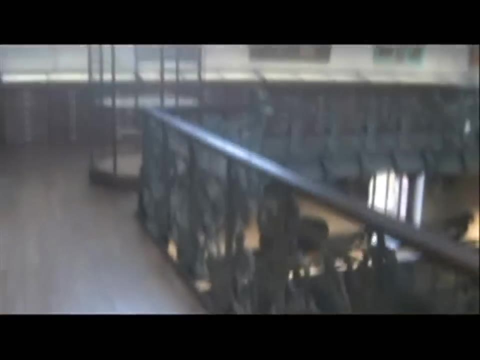 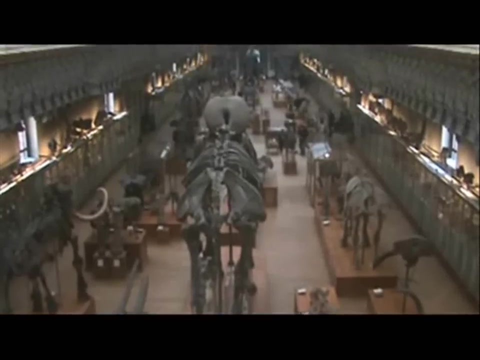 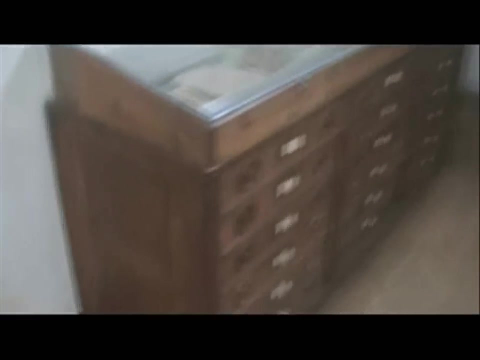 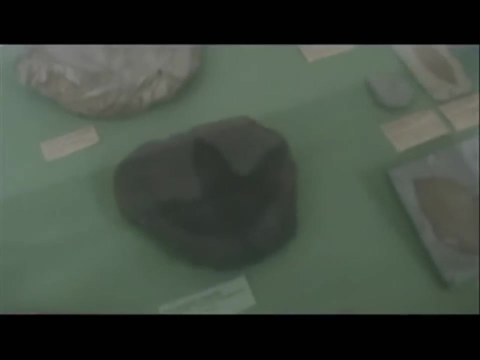 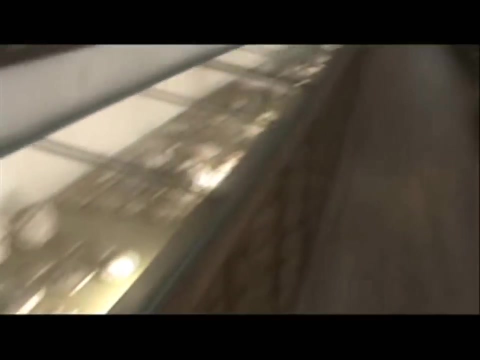 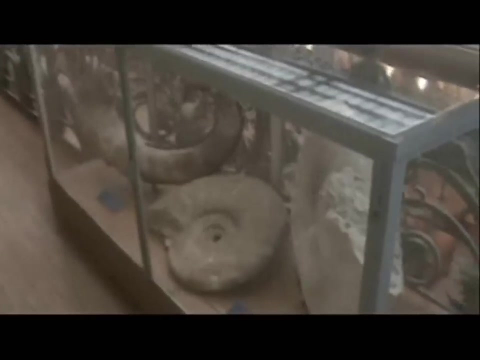 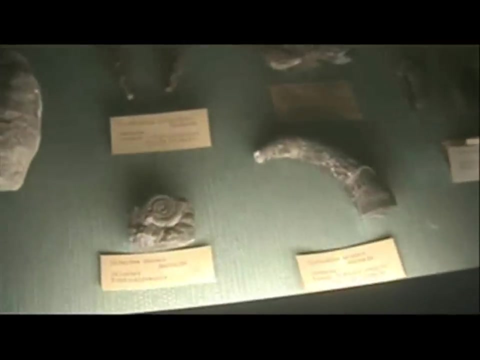 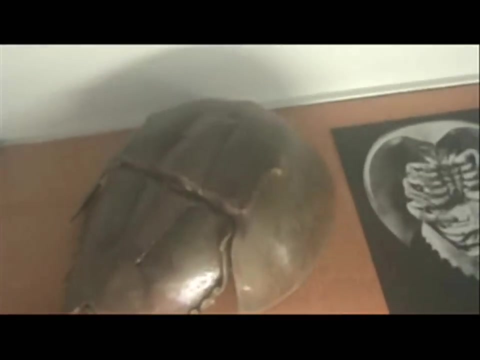 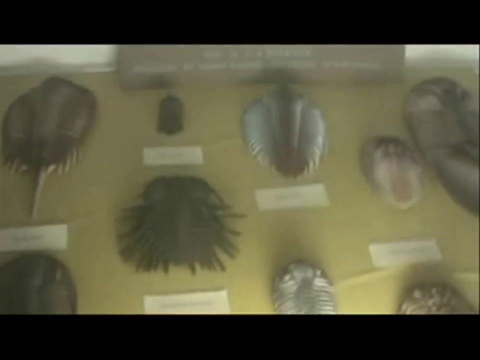 There's universities nearby too. This is definitely not the most popular area. See, it's one of those things about you know, going to places and exploring. you really find interesting places to find and go, you know. Alright, It's very fascinating stuff here actually. 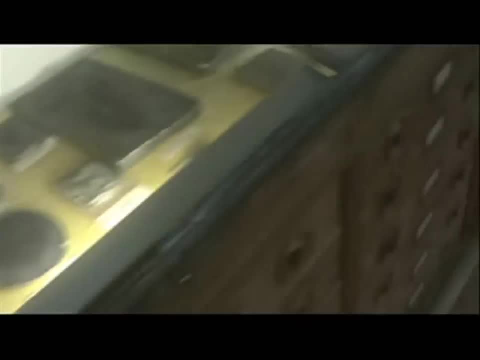 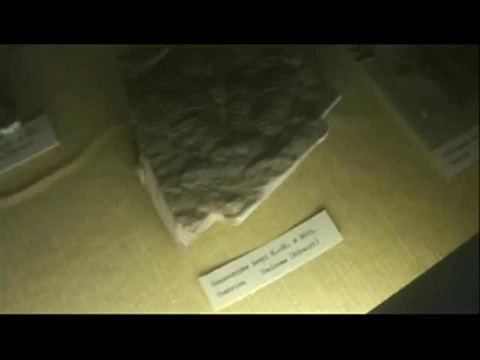 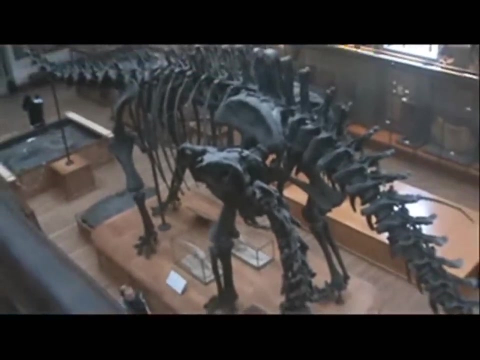 But you know, like I said, once you get to the top floor it's not. it's less creepy, Because then it's just like normal rare fossil that you could find in the right locations. It's a better view. 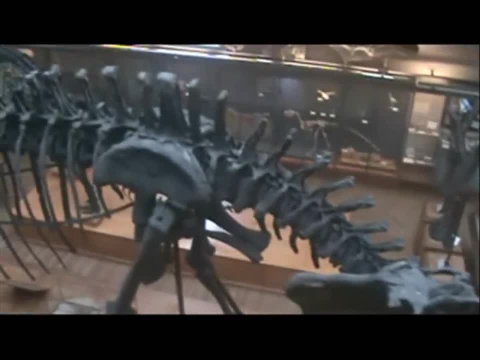 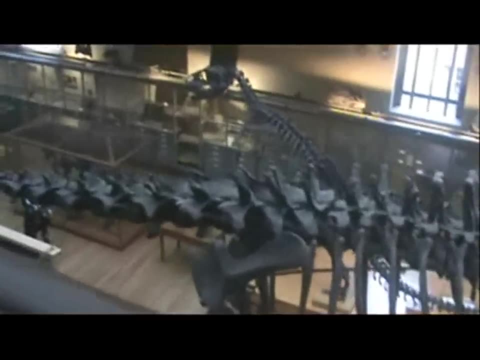 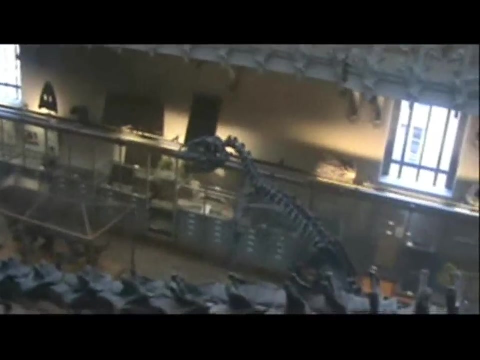 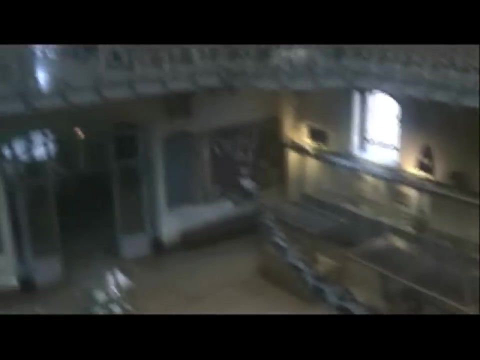 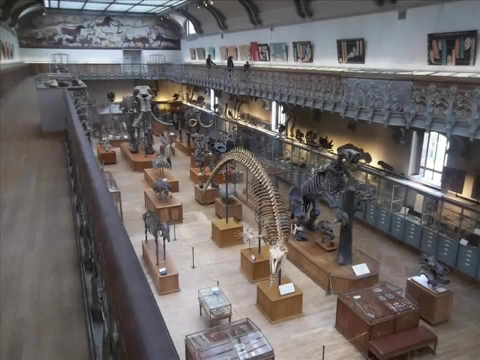 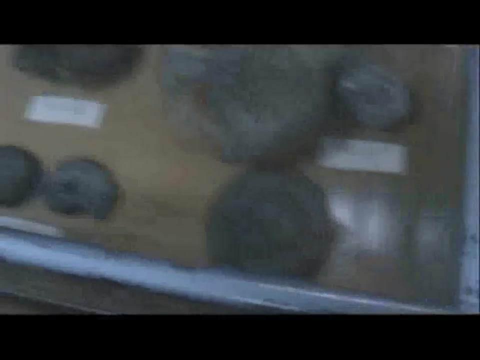 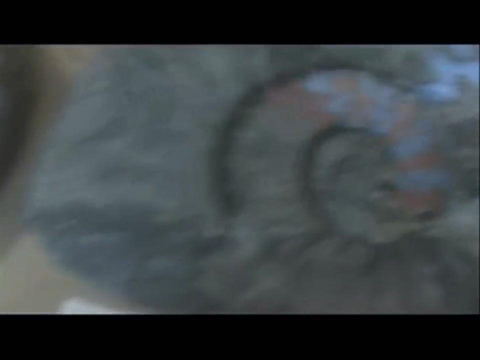 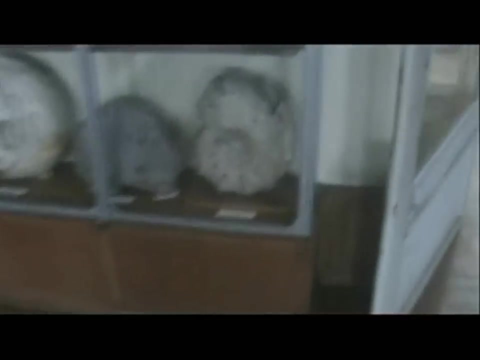 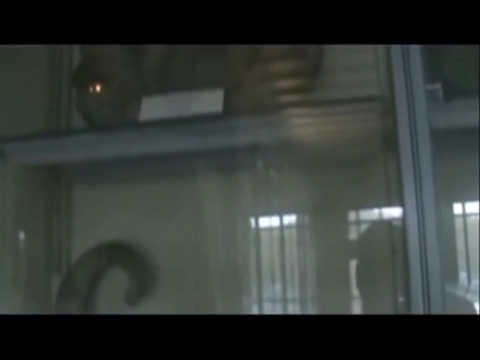 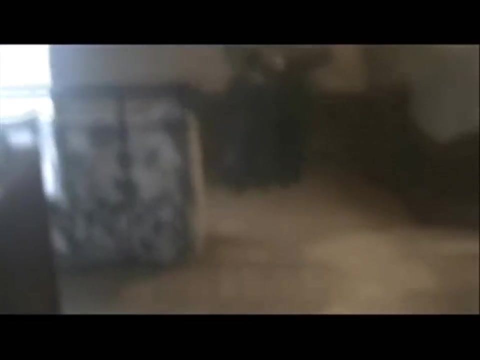 That was one big sucker. huh, Still more places to go. Yep, it was. There's some big ones over here too. You know, the museum doesn't look too big from the outside, but on the inside it's huge. 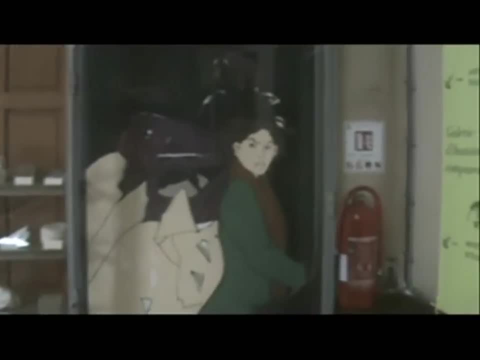 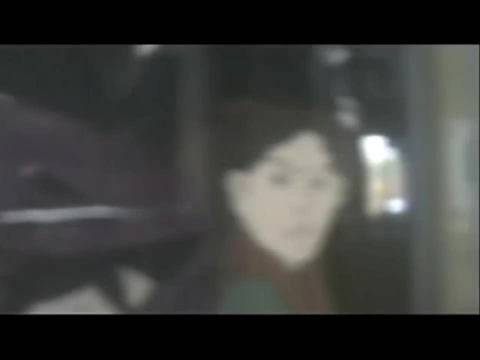 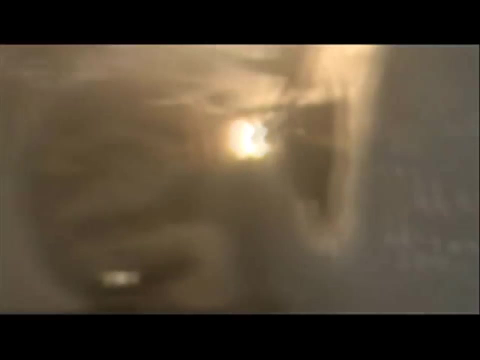 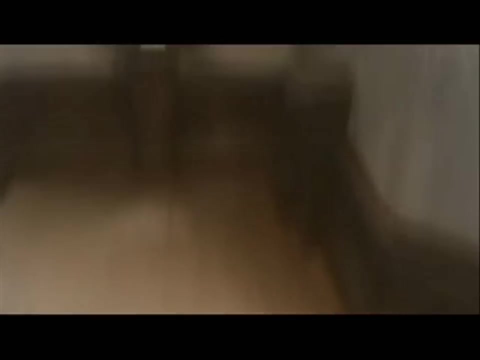 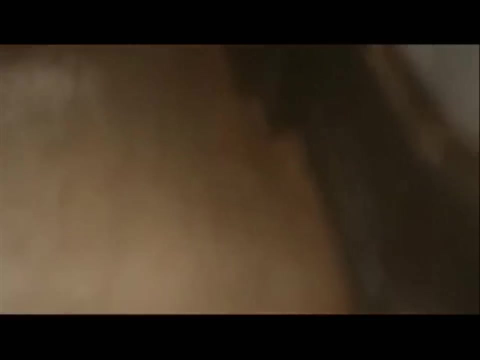 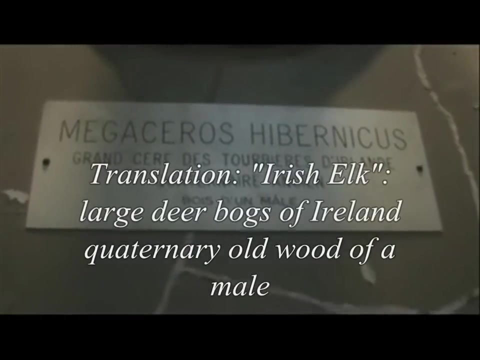 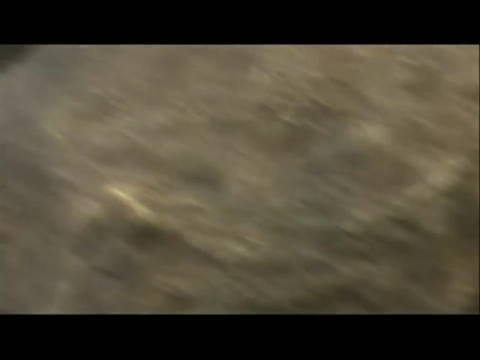 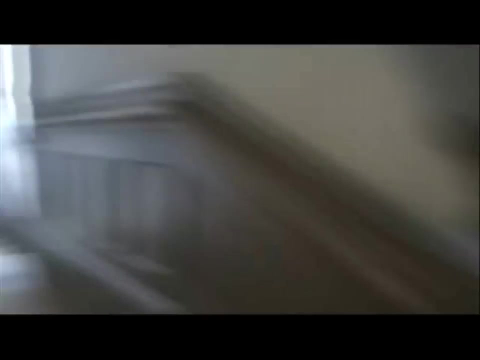 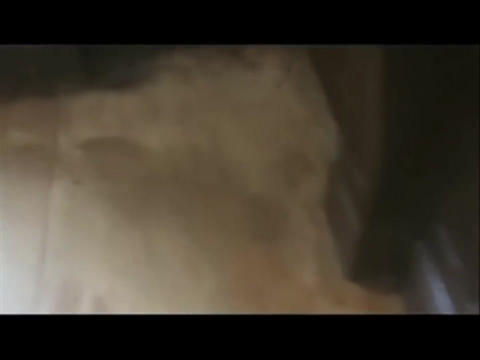 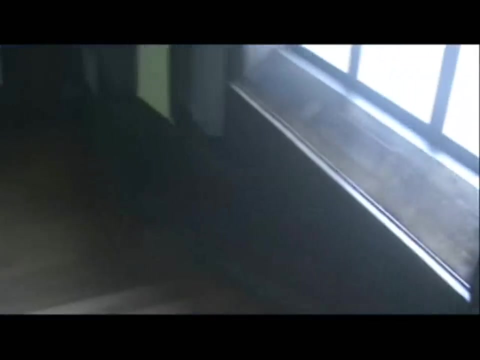 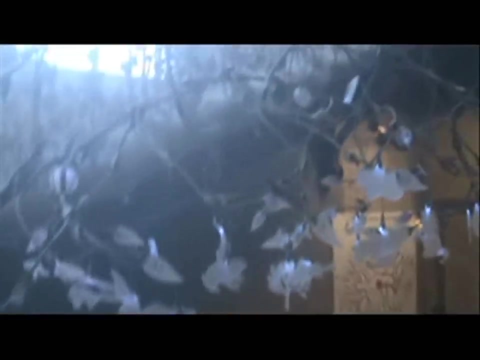 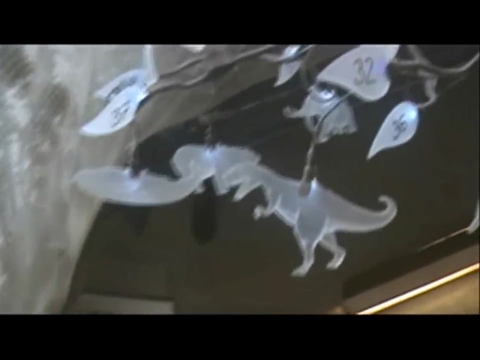 And is that Mary freaking Poppins? Or is that Mary Poppins and the dinosaur behind her? Okay, I don't get it. Hmm, still don't get it. Hmm, A little kind of new creepy chandelier for a lighting system. dinosaurs, whales, birds- oh, okay, I think you. 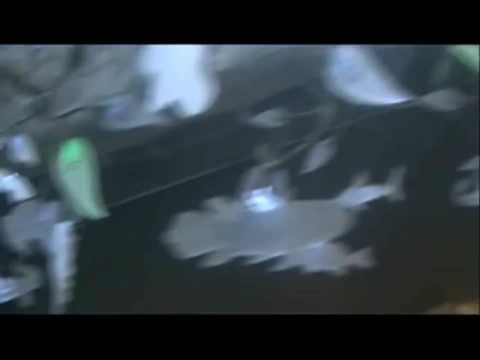 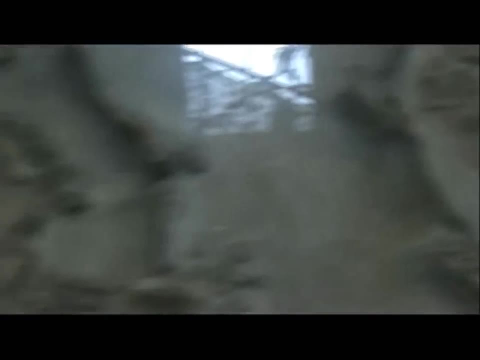 Oh, you can see the light up, Or whatever you know um, I don't know again. as I've said like a thousand times, I don't know French, so it doesn't really mean much. And if you ever get lost in place, usually that means the exit Man running.